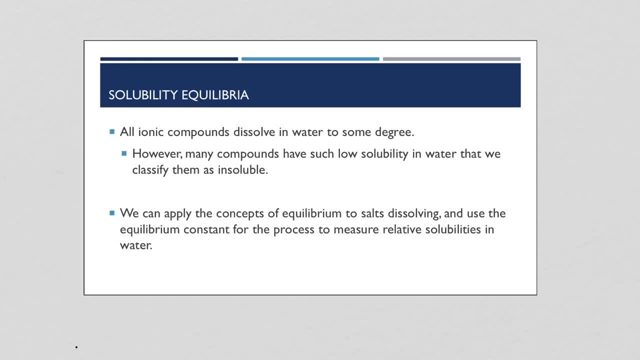 So you want to be working on the pre-lab, do an introduction, do a procedural flowchart, just like you would any other week for lab. One last comment about class procedures. We will be having normal Friday quizzes. They are now structured as talent quizzes. 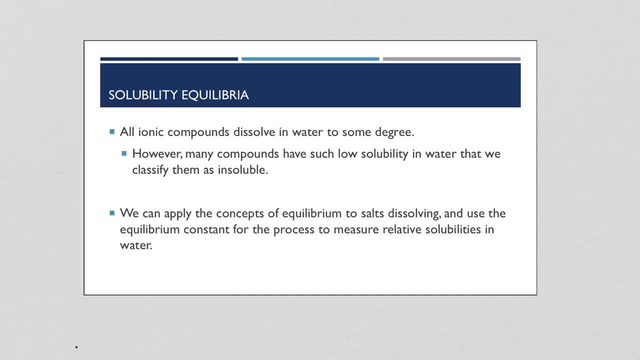 And so that quiz will become available on Friday morning- I think it's 7 am- And you will have all day, Friday, to take it. They are timed quizzes about 12 minutes or so, And you'll get one attempt, just like we were taking them in class. 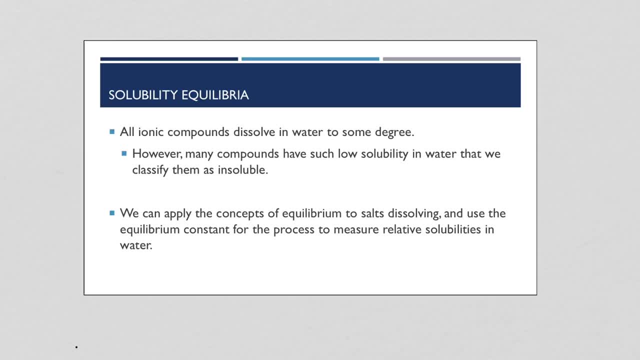 So you want to look in on talent under again, the Unit 3- and look for the Week 10 quiz And you want to make sure and complete that on Friday. So I hope everybody is surviving out there under these nice quarantine conditions. 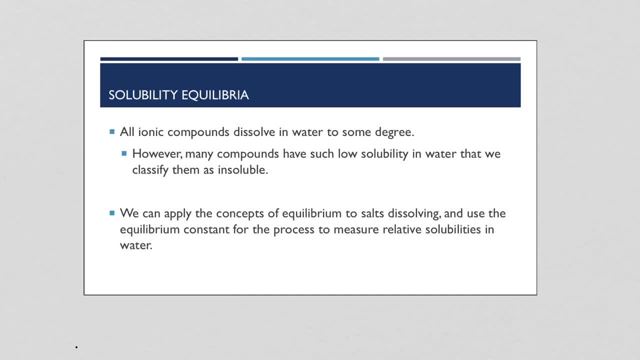 And hopefully having these videos will add a little bit of normalcy to this experience, as we try to get through this And learn some chemistry at the same time. So, again, today's topic: we're going to be talking about solubility, equilibrium. 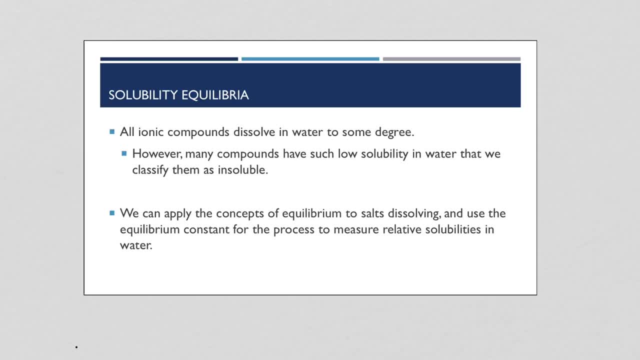 So continuing our discussions in Chapter 18.. Now, solubility equilibrium deals with a concept that we first talked about back in Chapter 5 in Chem 1, where you learned about solubility rules And we learned that all ionic compounds dissolve in water to some degree. 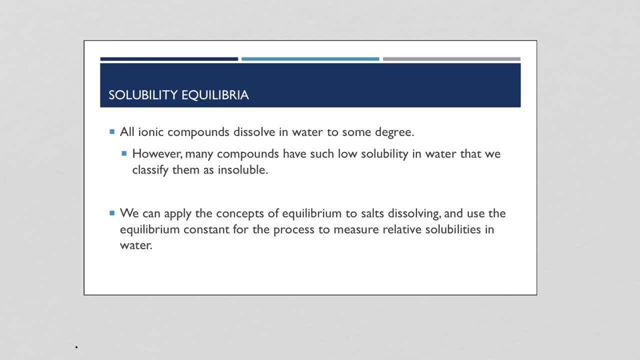 At that point we classified Things as either soluble or insoluble. But in reality some of those compounds that we call insoluble are really just very low solubility, very much imperceptible to just observing the solution. Then at the beginning of this semester we started talking about solutions and how those are homogeneous mixtures. 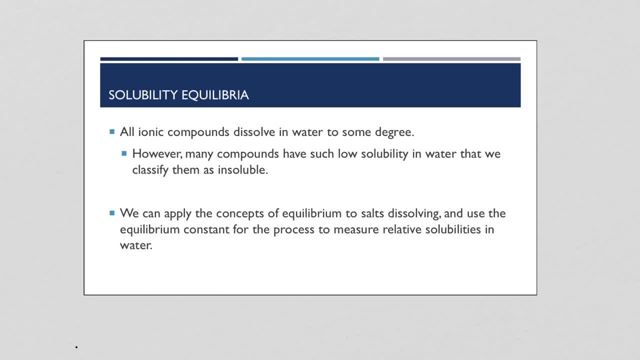 And, of course, one type of those solutions were dissolving a solid Into a liquid, So having a solid solute into our liquid solvent. So in this chapter, in this section, we're going to talk a little bit about the equilibrium that is present there between the dissolved solid. 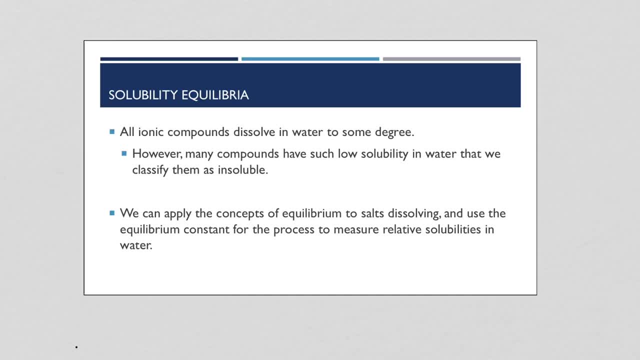 And the solid itself. So when the solid is added right, it initially will start to dissolve And then at some point an equilibrium develops Where the rate Of dissolving solid is equal to the rate of what we would call recrystallization, or coming back out of solution. 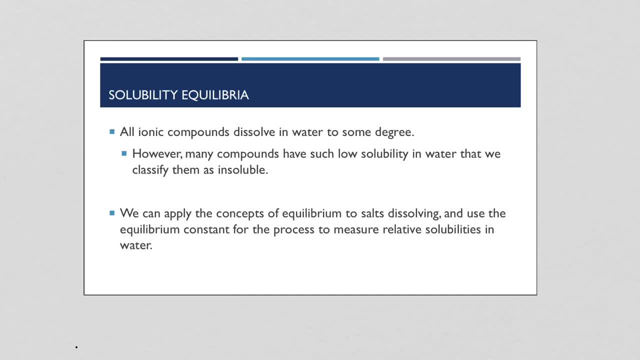 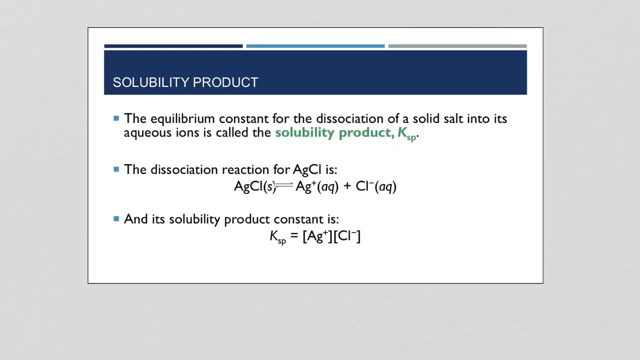 And so that's the equilibrium that we're going to be exploring in this section, So we can apply all the same concepts that we have to other kinds of equilibrium That we to this solubility equilibrium, So the equilibrium constant for the dissociation of a solid 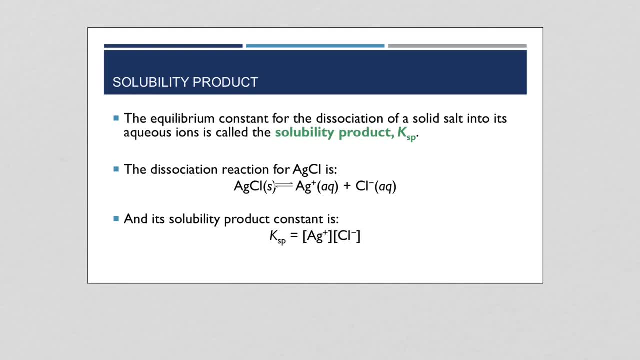 Into the aqueous ion is called the solubility product constant or KSP. So this describes the equilibrium here between the solid And the dissolved ions, And notice of course the equilibrium arrow Indicating There is a balance there between the rate of dissolving. 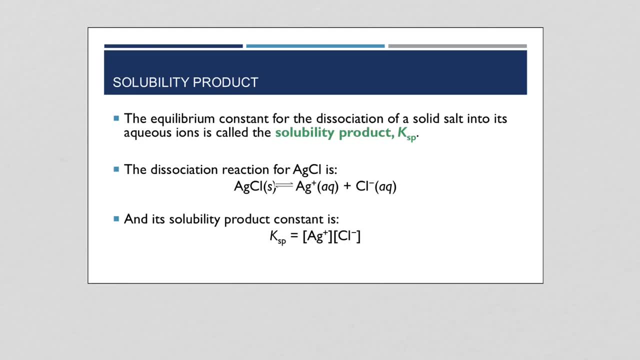 And recrystallization. Now we can express the equilibrium expression, right, the KSP expression, As normal with our products Over our reactants. And so in this case, right, The reactant is a solid, So of course it won't be included in our equilibrium expression. 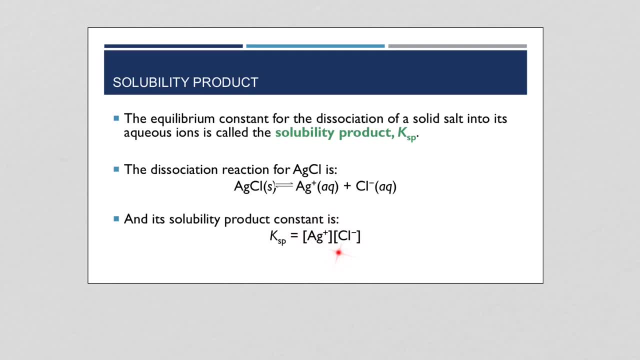 So it ends up Only being the product Of the ion concentrations, Or our products here. So for the example listed here, We would have the solubility Of the silver ion Times, The concentration of the chloride ion. Now, of course, these concentrations are going to be related by the stoichiometry. 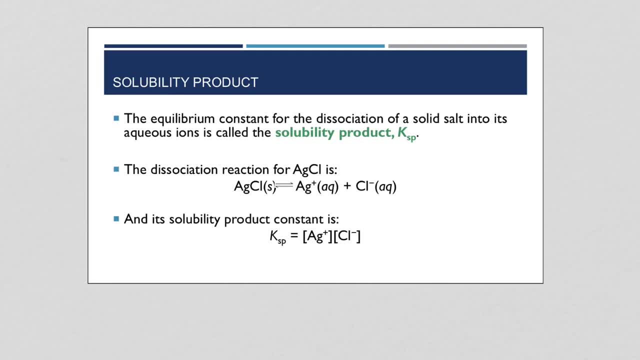 Of our initial Compound. So in this case, with silver chloride, We have a one to one stoichiometry, So We're going to get equal amounts Of silver ion And chloride ion. So these two values right are going to be the same. 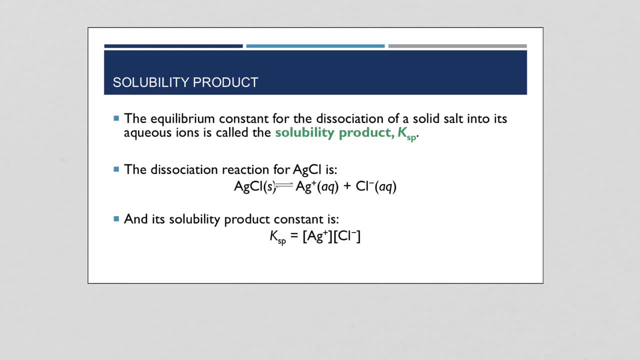 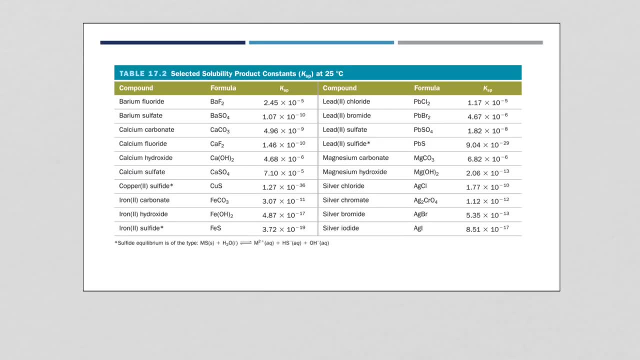 We're going to create The same number of silver ions as we do chloride ion, So one to one stoichiometry. Now if we look at this table real quick here, We can see that there's a huge range Of these KSP values. 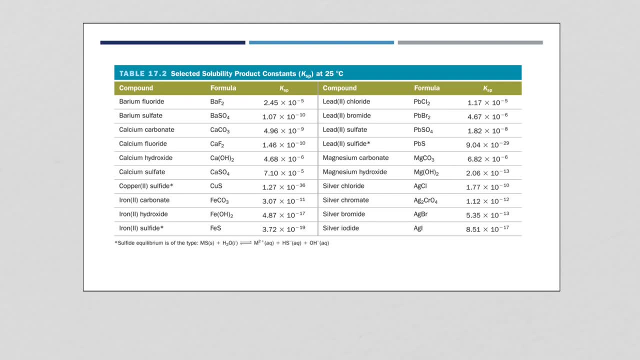 And remember from our general discussion of equilibrium, The bigger that number is, The more product favored. So in this case, right The more soluble, right The more it favors the dissolved compound, So things that we would commonly associate as being soluble. 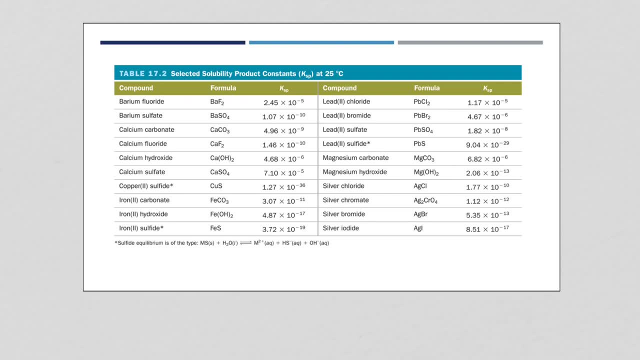 Something like barium fluoride Or Calcium sulfate here. Right, These are going to have fairly Large, if you will, Solubility products. Now, this table is just obviously a sample list, And most of these Are Even the ones that have fairly. 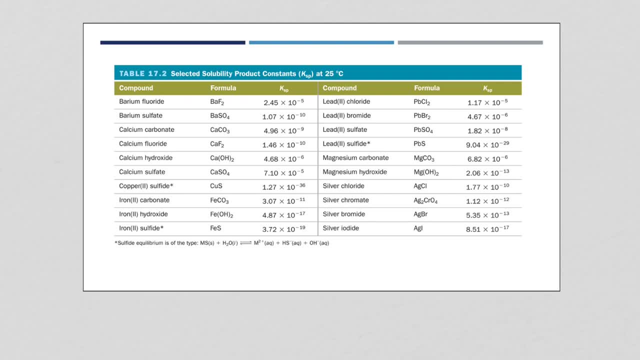 High values are still fairly low solubility, But we can go to extremes here and see Things like Silver iodide, Silver chloride, Silver bromide. These have Really small solubility. These are things that, If we were classifying them on our solubility table, 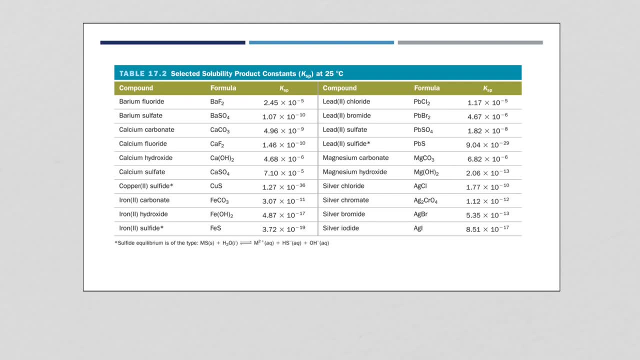 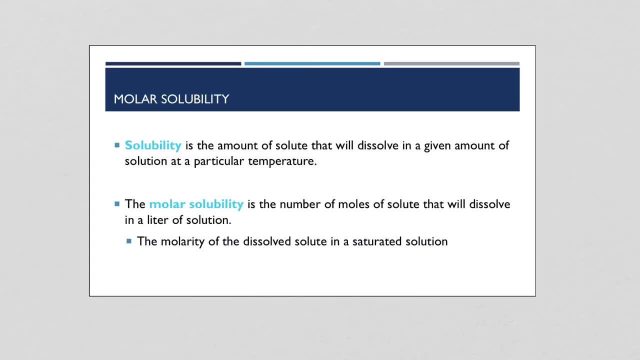 We would classify them as insoluble. They don't dissolve at all. Now The vocabulary here. When we use the term solubility in this context, We're talking about The amount of solute that will dissolve in a given amount of solution at a particular temperature. 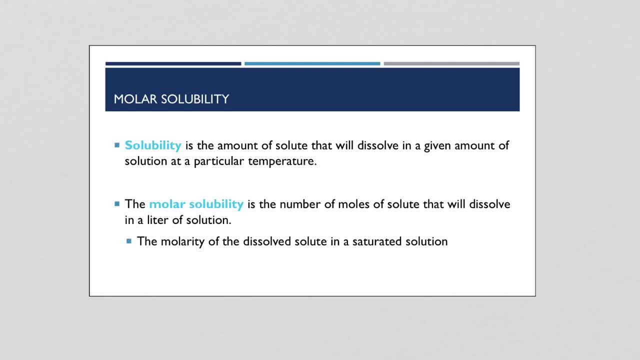 We've introduced this term in an earlier chapter, And this is how we quantify the amount Of solute that is dissolving. Now, Another way to express that Is in something called the molar solubility, Which is The number of moles of solute. 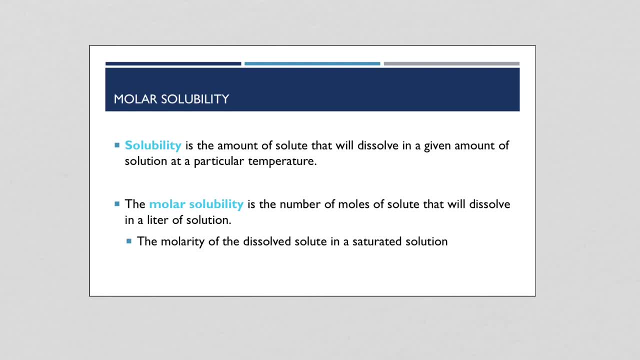 That will dissolve in a given liter. Now this may seem Quite familiar to you, Because If we remember the moles of solute Per liter of solution Is simply the molarity, So the molar solubility Is. 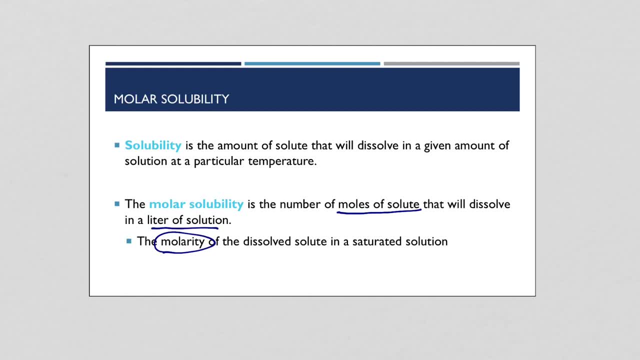 Expressed as a molarity, The number of moles that will dissolve In a given liter Of solution. And this is a very common way That we express The solubility. In this context, Right, We express it as: 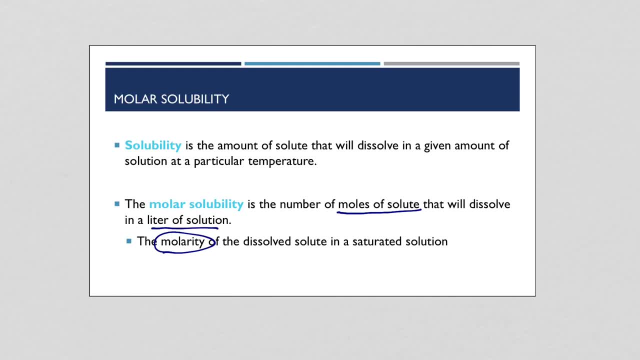 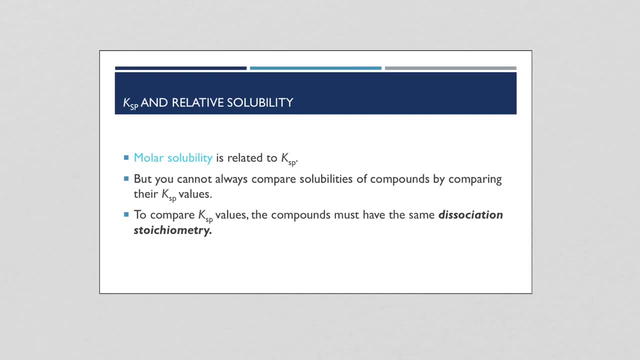 The molarity. Now, the molar solubility is of course related To the KSP value, But We have to be careful In comparing these. So If we remember from our previous slide That The Example for silver chloride 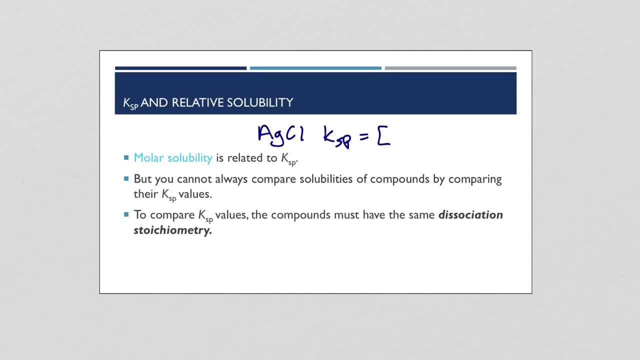 The KSP value is equal to The solubility Of silver ion Times the chloride ion. So each of these values would be The molar solubility Of that ion Right Now, One thing we have to be a little bit careful of. 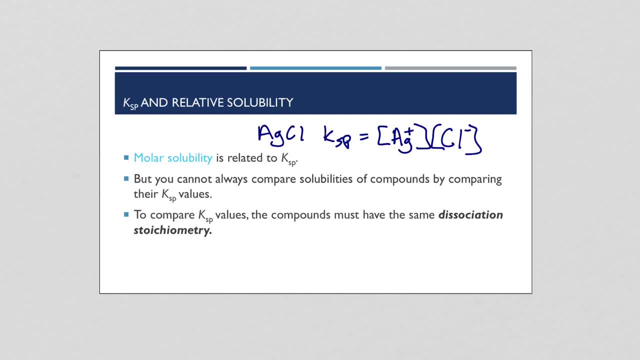 Is We can't just Look at The KSP values In order to compare solubility. So, For example, We can't just look at any two compounds and say, Oh, This one is going to be more soluble than that one. 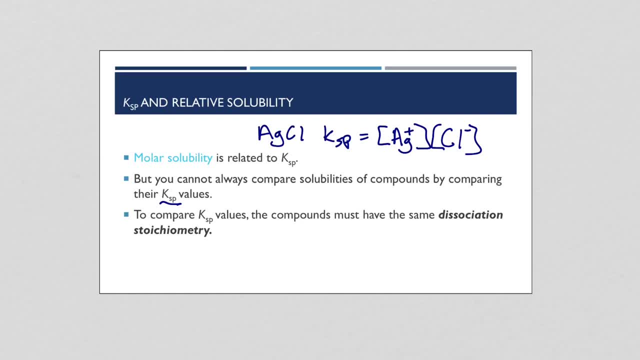 Because it has A larger KSP value. We have to make sure that we're comparing things That have the same Dissociation Stoichiometry. Now, what that means is We could compare something like Silver chloride, To say. 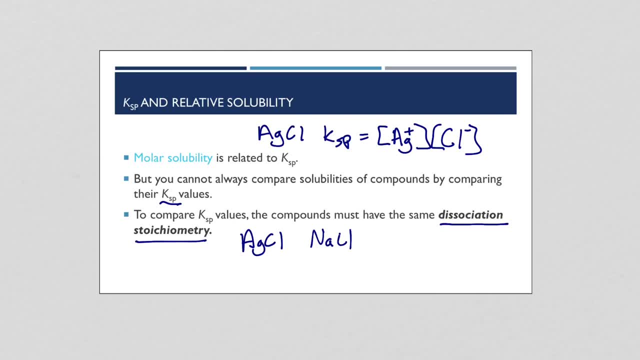 Sodium chloride, Because they both have a one to one stoichiometry. But We wouldn't want to compare Silver chloride And sodium chloride. We wouldn't want to compare it to something like Magnesium chloride, Because we have a different. 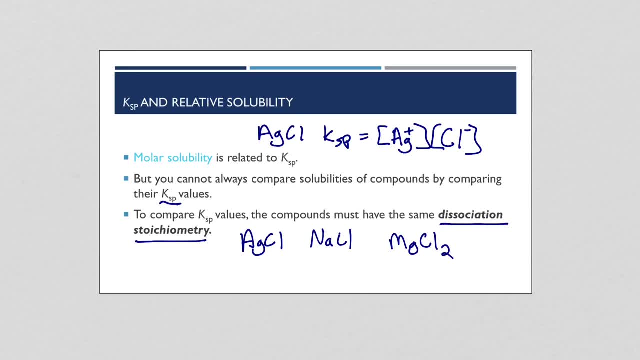 Stoichiometry. here We have a one to two stoichiometry, So for magnesium chloride It's KSP Right Is going to be equal to Magnesium, But the chloride ion Right Would end up being squared. So 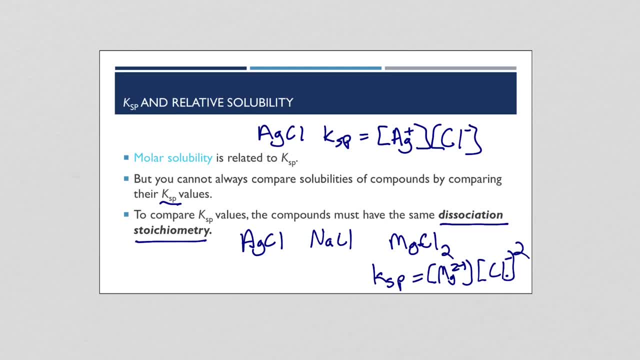 We can't compare this KSP To the KSP For silver chloride, So we don't want to compare this value To this value To give us a measure of Solubility Right, Because we have a different stoichiometry. 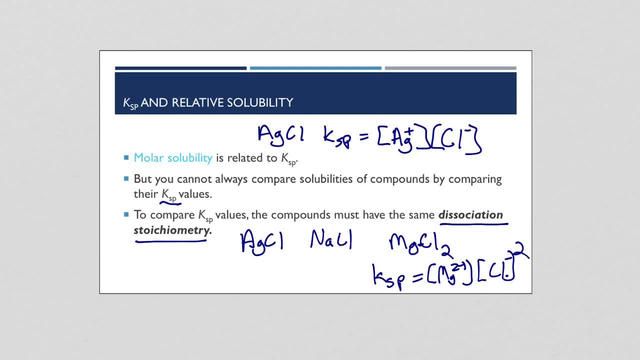 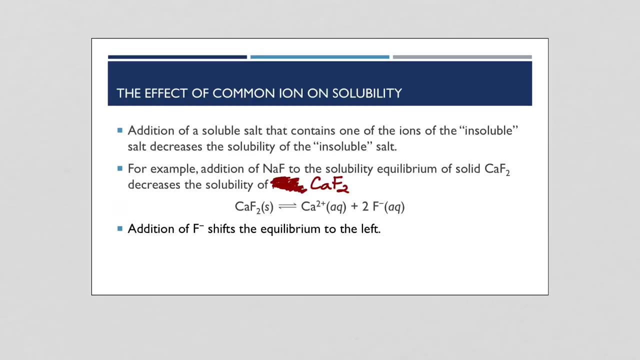 So we just have to be careful To look at the stoichiometry If we want to make direct comparisons Or use KSP to predict If one material is more soluble than another. So the next effect that I want to talk about: 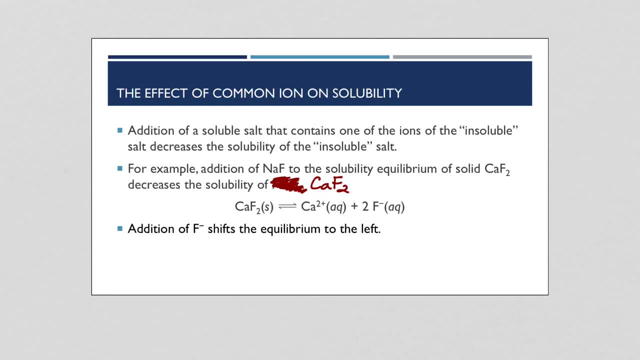 Is the common ion effect. So we saw this When we talked about buffer solutions, Where having that common ion, Or what we would call the conjugate base, Present Reduced The ionization of our acid. That's lowering the Raising the pH. 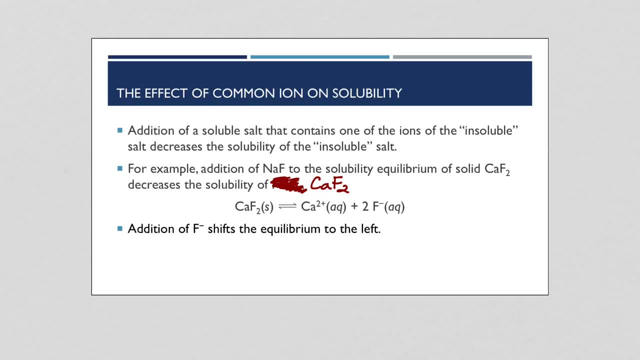 Making the buffer solution Less acidic than it would be If we had just added that same acid To water, With none of that Or no additional Of that conjugate base Or common ion Present in solution. Well, we can see the same effect. 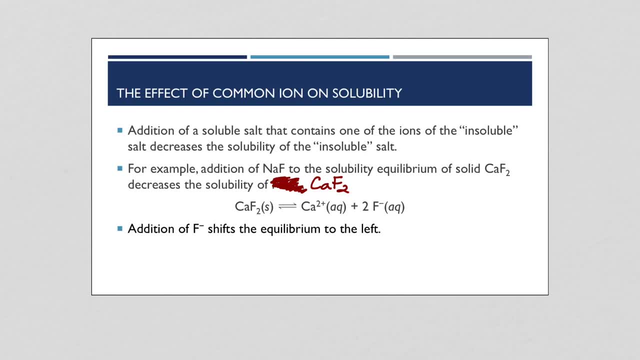 When we talked about the solubility of ionic compounds. If we, instead of adding An ionic compound to simply water, We added to a solution that already contains One of the ions In our salt, Then we will change the solubility. 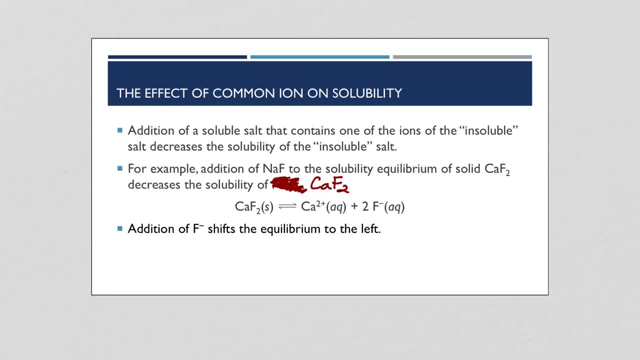 So, for example, If we added calcium fluoride To a solution that already contained sodium fluoride, Or in other words, already contained Some fluoride ion, That's going to alter the solubility. So if we look at the solubility expression, 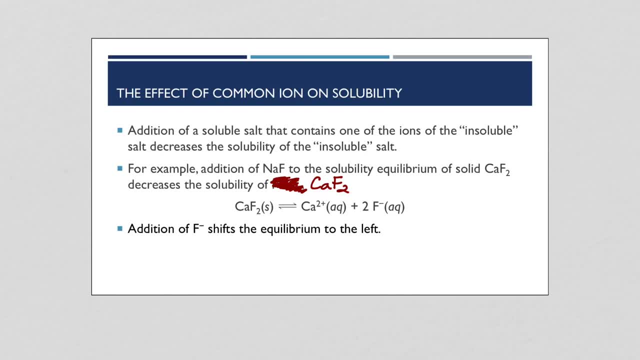 Here For calcium fluoride, Breaking down to calcium ion And two fluoride ions If we already have F ion present Right. Le Chatelier's principle, If we remember, Is going to shift The equilibrium To the left right. 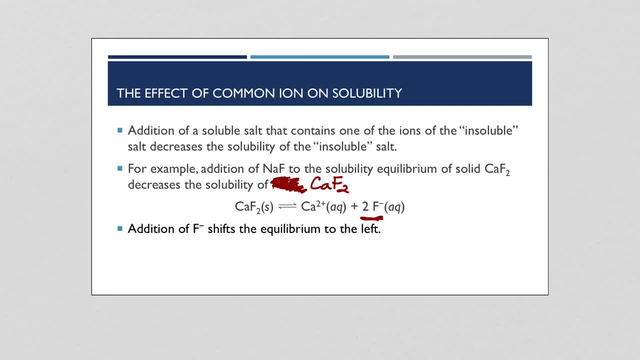 So if I already have More of this present, That's going to shift the equilibrium to the left And it's going to reduce The solubility Of the calcium fluoride. So having that common ion effect Will ultimately lower the solubility. 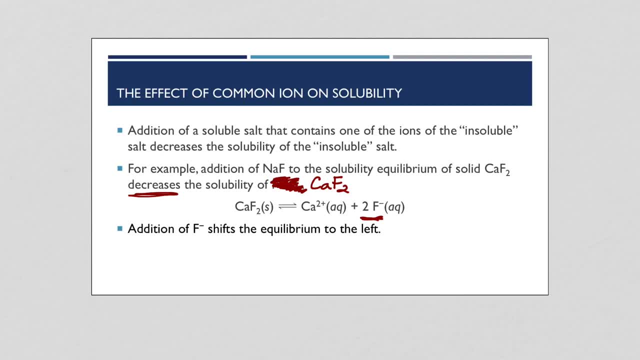 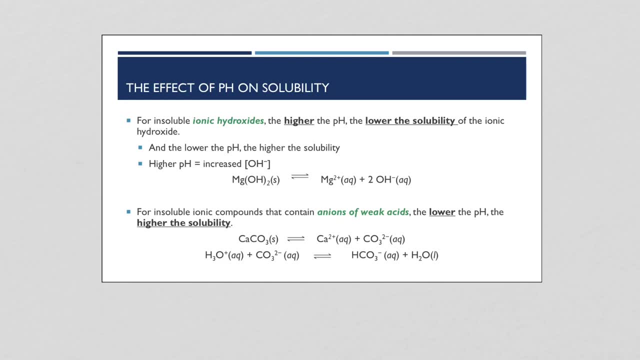 Of the salt that we're trying to dissolve. Now, the pH of a solution Will also have an effect On the solubility, Just like we saw with the common ion. Now, the general effect here Is that The more acidic. 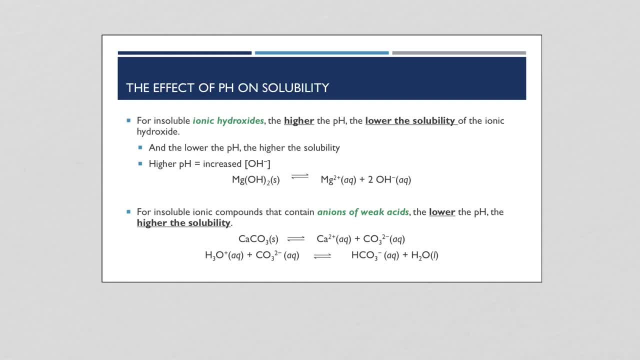 The solution, The higher the solubility Will be for most Compounds Or most ionic compounds. So we can look at a couple examples. First of all, we can look at Ionic hydroxides, Which tend to be: 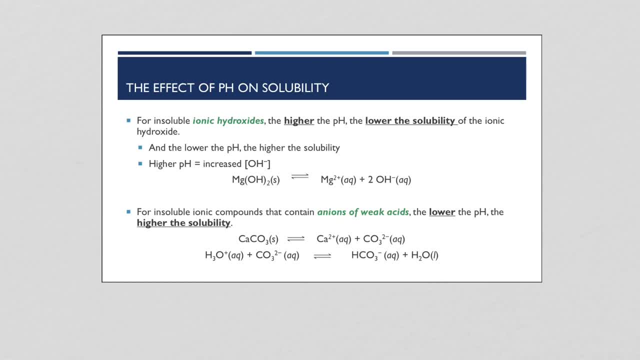 Insoluble, Such as Magnesium hydroxide, Aluminum hydroxide. They tend to have sort of a lower solubility. But If we Lower the pH Right, Make it more acidic, We increase the solubility. 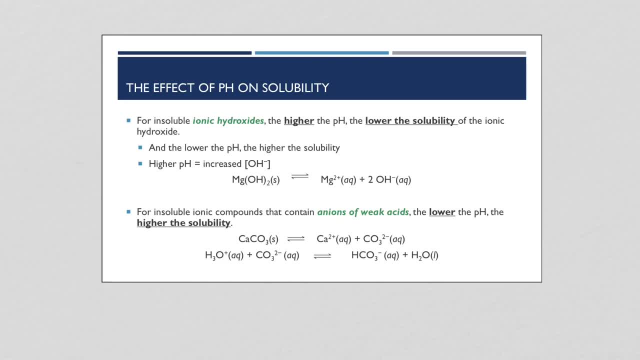 And at the same time, of course, The higher the pH, The more basic the solution is, The lower the solubility. So as the solution becomes more basic, They become less and less Soluble. If we look at the equilibrium, 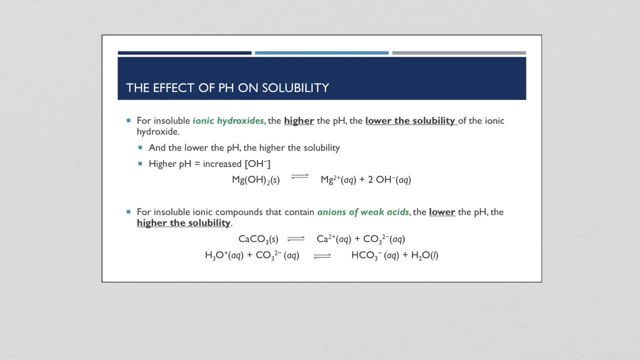 Here we can see that We have Magnesium hydroxide In equilibrium with its ions, So this has a fairly Low solubility, But We can see at high pH, In other words, More hydroxide ion. 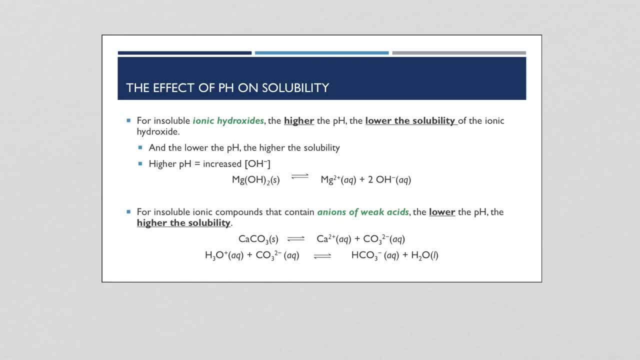 Le Chatelier is going to push That equilibrium Back To the left At high pH. Now, If you Lower the pH, Right, You're going to have a less hydroxide, Right, You know, More hydronium. 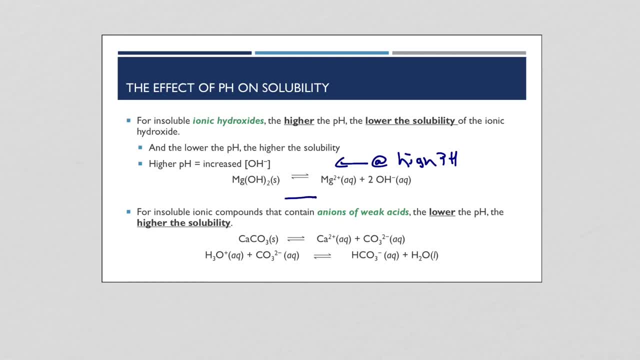 That's going to tend To push the equilibrium Again To the right At low pH, And so That's going to increase the solubility. So the net effect is For these hydroxides Is going to be: 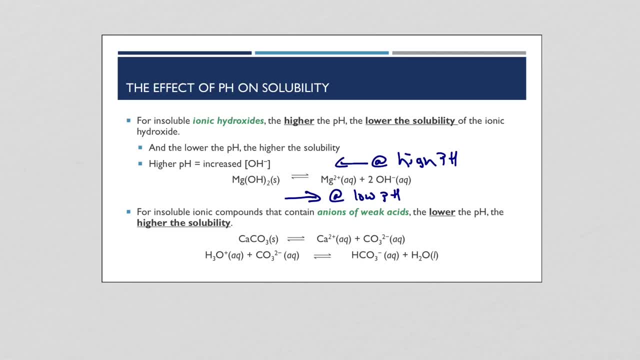 An increased solubility At lower pHs Or more acidic conditions. Now we can also see that Even if The anion present Is not the anion of a strong base, Right If it's the anion Associated. 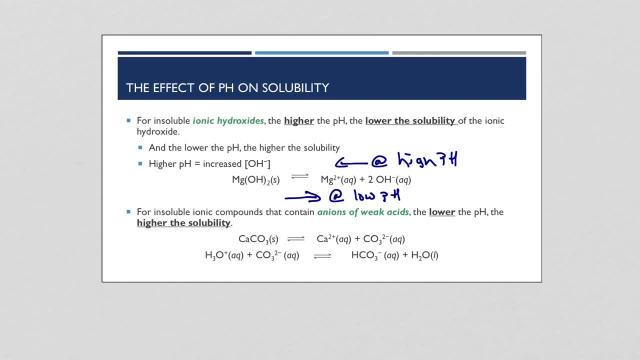 With a weak base, Or in other words The conjugate ion Of a weak acid. So carbonates Are a really common example Right Of this. And so If we have calcium carbonates, Equilibrium with calcium carbonate. 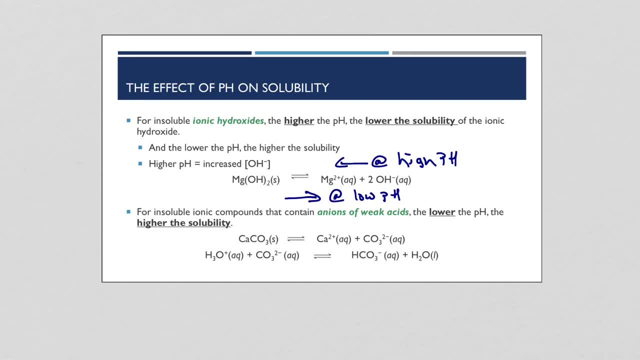 Carbonates are notoriously Low solubility materials, But If we Increase the acidity Right, In other words, If we have An ion, That hydronium ion Is going to react With the carbonate ion Here. 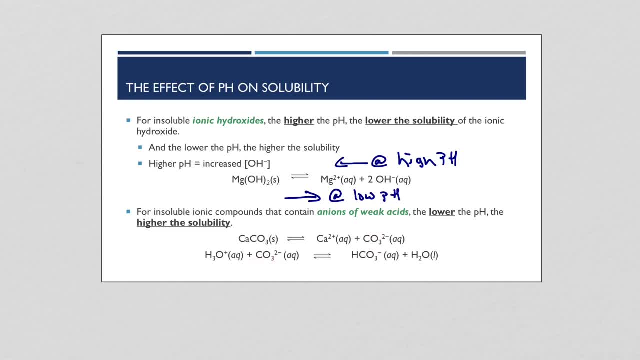 So that hydronium Is going to react With the carbonate ion That we have here And produce, In this case, Bicarbonate and water. But the net effect is We're going to be Removing The carbonate ion. 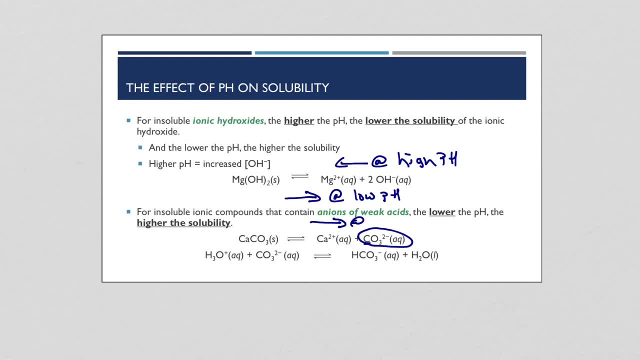 And Push our equilibrium To the right At low pH, Or, in other words, It's going to make Our carbonate More soluble, Because our product here, Our carbonate ion, Is being used by the Hydronium ion in solution. 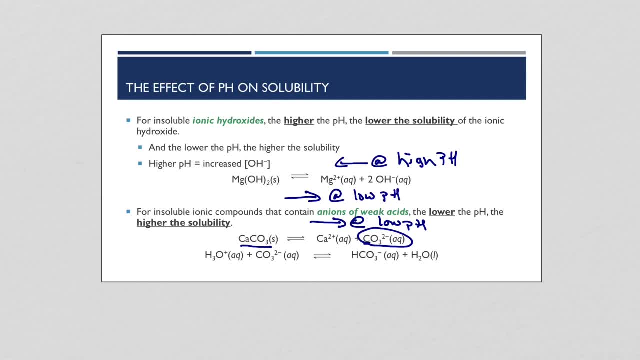 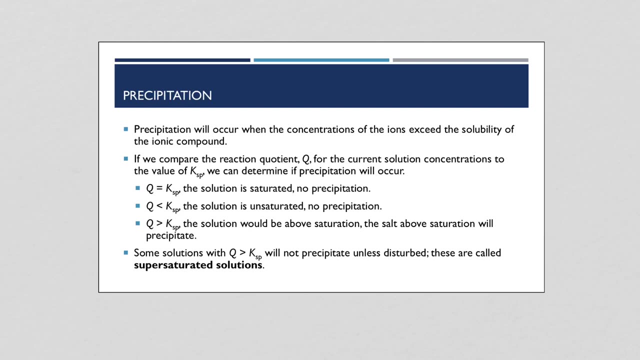 In the more acidic conditions, Which is then going to Pull the carbonate Into solution. So the last topic That I want to talk about In this section Is precipitation. So we're all familiar with Precipitation from Chem 1.. 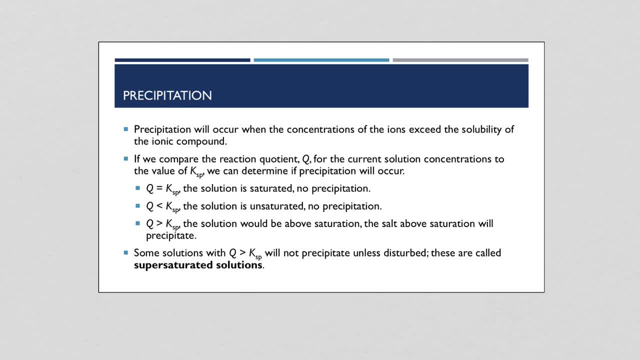 Where we talked about Precipitation reactions Of ion With dissolved ionic compounds, And two of the ions present Can combine To make something. To combine to give us an ionic compound That is insoluble According to our solubility rules. 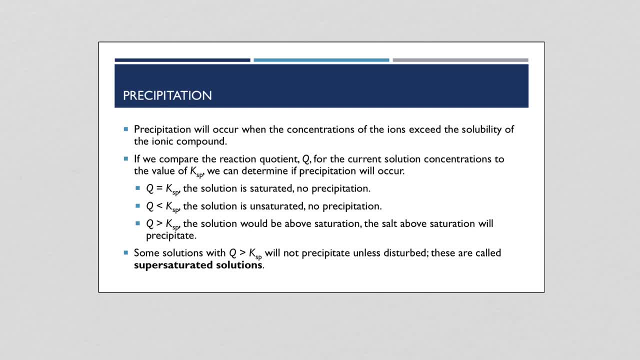 Or, as we see now, Meaning it has a very low Ksp value, Then it will precipitate Out of solution. Now we can dive into that Just a little more deeply, The solubility Equilibrium, And look at 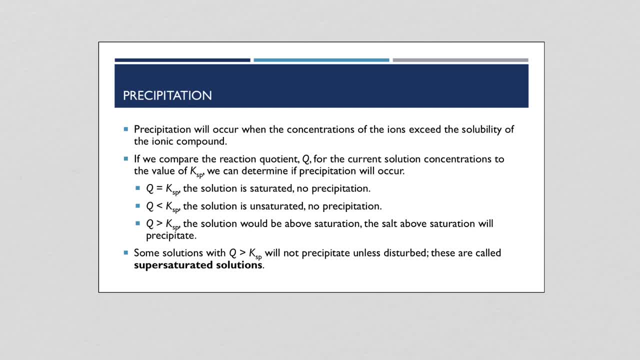 What does it mean For that precipitation to occur? We also introduced The terms Saturated, Unsaturated And supersaturated Or above saturation Earlier, And We knew that something precipitates When we get Above the saturation. 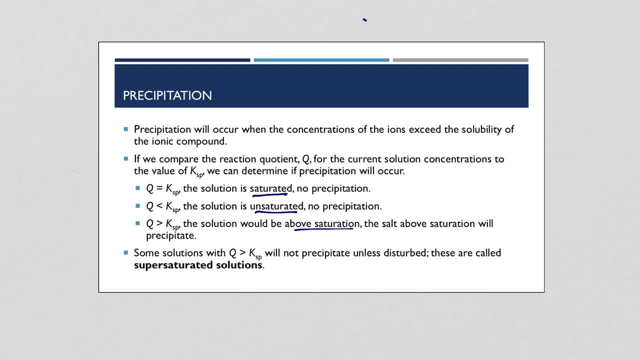 So unsaturated Simply meant we were below The solubility maximum, For that Saturated means we were at that solubility Maximum, The most that we can dissolve, And if we were above the saturation, Or something called supersaturated, 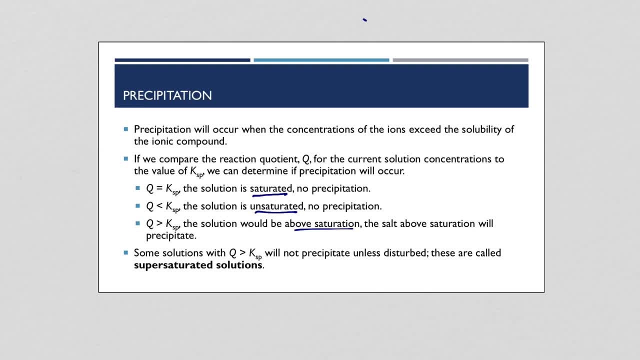 Then We would start to precipitate out. So that's what we're going to see here, Right, But how can we use KSP to help us? Well, We're going to rely back on something we learned Back in chapter 16.. 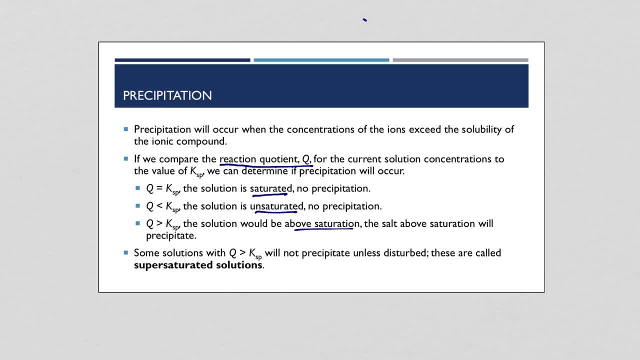 When we first talked about equilibrium, And that is the reaction quotient, Or Q, Which is just simply solving The equilibrium expression Products over reactants, But at non-equilibrium conditions. So In this case We're going to use the concentrations. 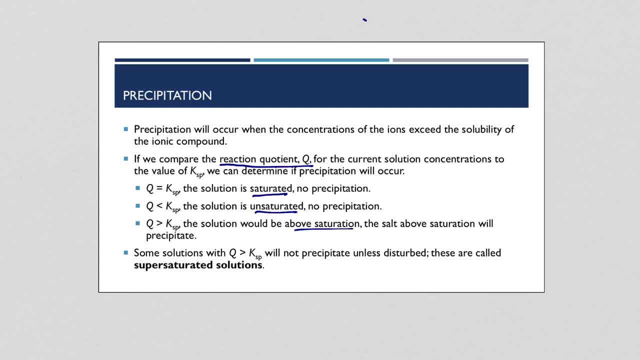 Of our ions Under whatever the current concentrations are. We're going to calculate our Q And then compare that, of course, To KSP, And we have three possibilities, Right? If Q is equal to KSP, Then we're saturated. 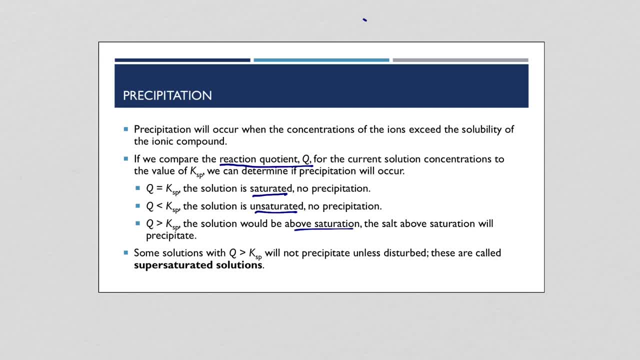 We're at equilibrium. That's what the saturation point tells us. That's when we're going to be at equilibrium. If Q is less than KSP, Then we're at conditions, Unsaturated And equilibrium, If we want to think about it. 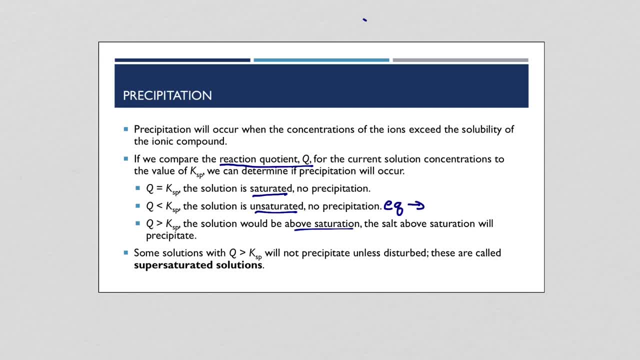 The equilibrium Is going to move To the right. To get to equilibrium Right, So Our reaction is going to move to the right Until we reach The equilibrium, Or try to If there's solid available to dissolve. However, 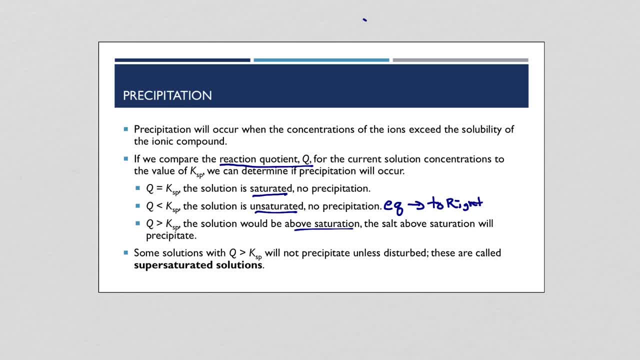 If we're at a condition Where our Q Is greater than KSP, That means that We have too much Or higher than the saturation point Dissolved in solution. That's going to trigger a precipitation. So if we create conditions, 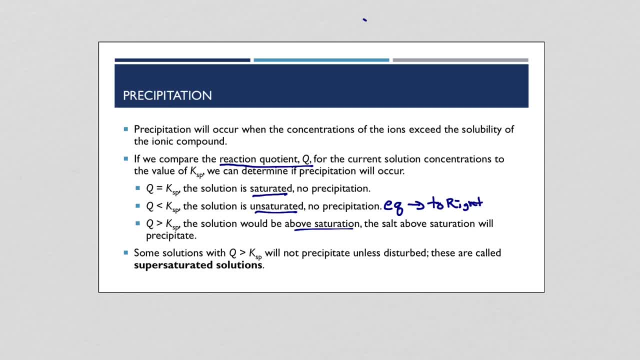 Where Q is greater than KSP. That's where We're going to see the precipitation And we're going to create The precipitate. Now Some solutions are more stable Than others, So we talked about In earlier chapters. 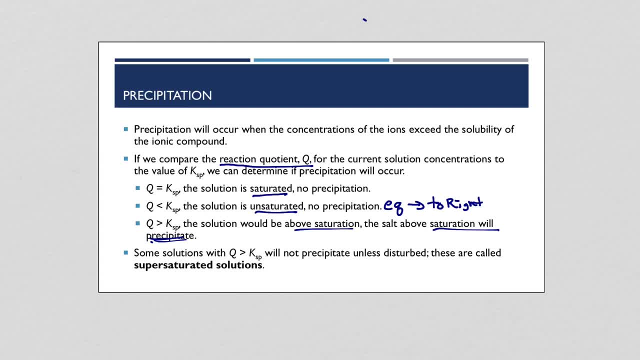 About creating supersaturated solution. These are typically able to be created Where Some solutions Are more stable, in solution Where Q is greater than KSP, But we don't see immediate precipitation For materials that can do that. They're able to create supersaturated. 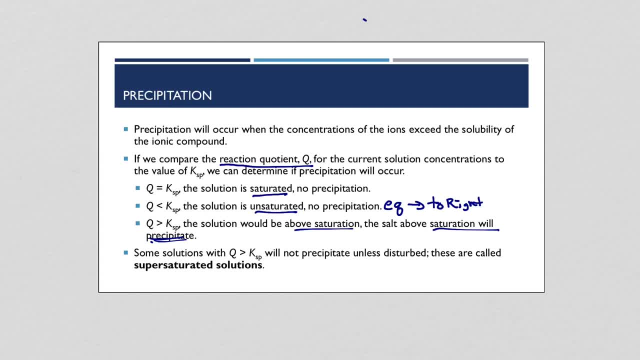 Solutions. But in most materials, As soon as you go above that solubility limit, You're going to start to see precipitation, Just like we saw When we talked about precipitation reactions. So When the solubility gets higher Than what it is at the saturation point, 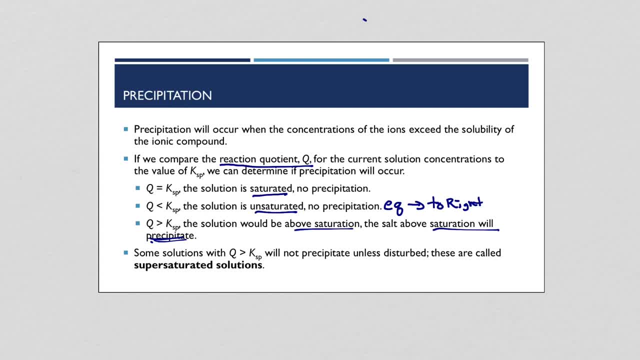 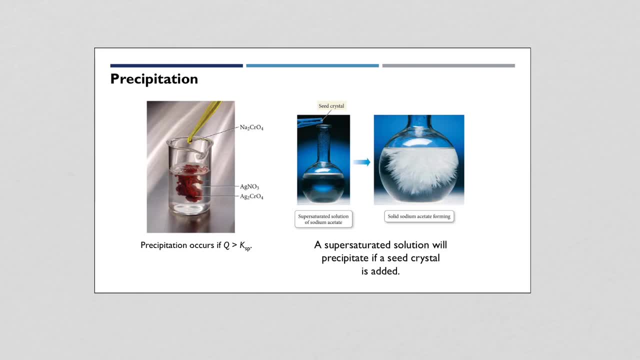 That tells me We're going to see precipitation. So, for example, If I Add a solution Of sodium chromate And Silver nitrate, I can Create A precipitate Of silver chromate, Because Silver chromate has. 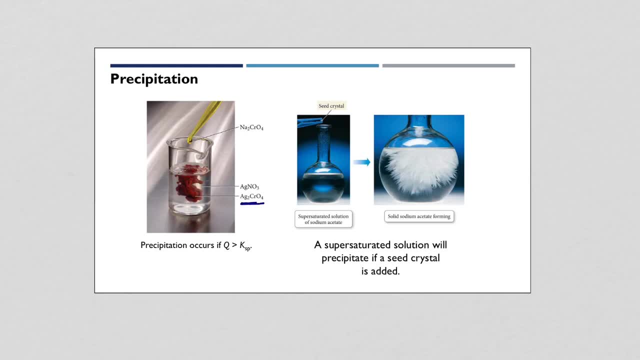 A very low solubility And with this, Sodium acetate Can precipitate. Now, Just to show you, Sodium acetate Is one of these solutions That is fairly stable As a supersaturated solution, So you can create. 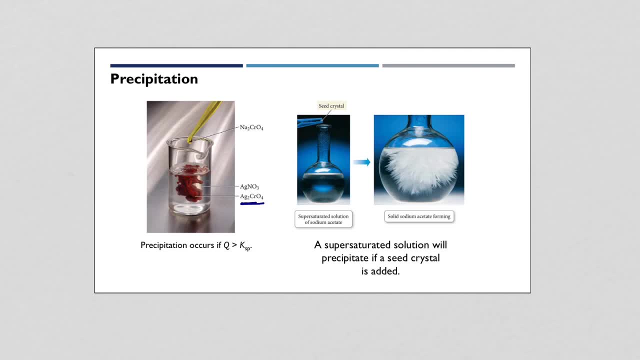 A supersaturated solution Of sodium acetate Without it precipitating. But if we disturb that in any way, Shaking it, You immediately start to see Rapid precipitation And sometimes you get quite Pretty displays Of crystallization To occur. 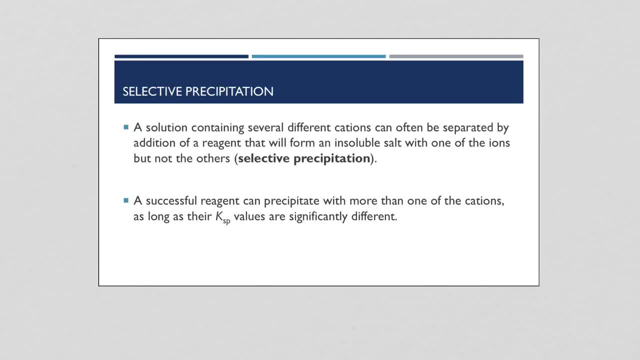 Now We can also use this Sometimes To do what's called selective precipitation. So this would be a situation Where we have multiple Different cations Or metal ions In solution That maybe we want to selectively remove One of the metal ions from solution. 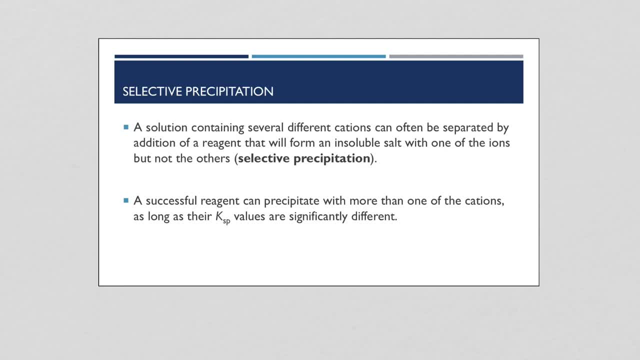 But not the others. So what we can do, then, Is we can add A material That has a negative ion That will pair With that positive ion And with one of the positive ions. It will create a solution. It will create a material. 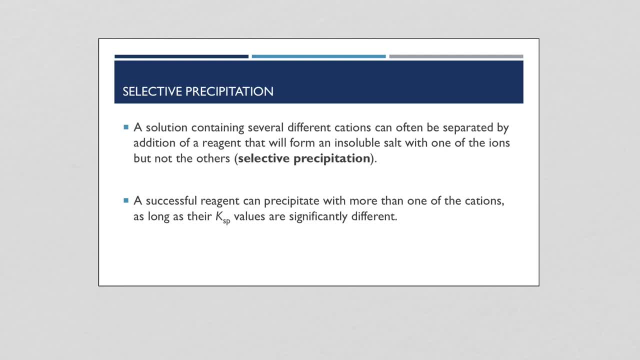 That has a very low solubility. With the other Cation It creates a salt, An ionic compound That has a higher solubility, And so one of those materials, The one with the lower solubility, Will precipitate out first. 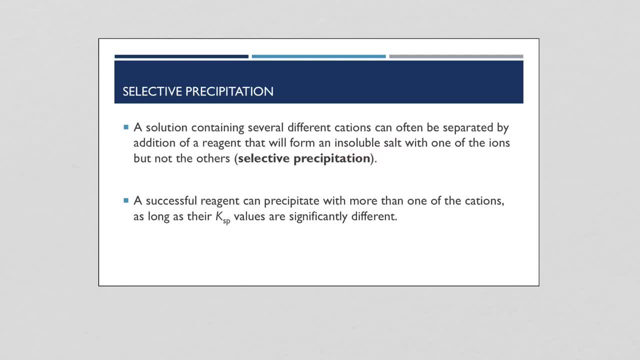 So it will form an insoluble salt With one of the materials Or with one of the positive ions, But not the others. So A successful negative ion Here We can precipitate With more than one of the cations. 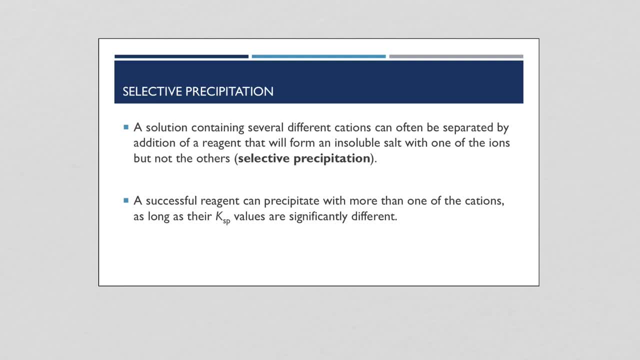 You know, Even if we have, say, three in there And maybe precipitate with two And leave one behind, The key is their KSP's Have to be significantly different. So Several orders of magnitude Difference Is typically What we usually look for. 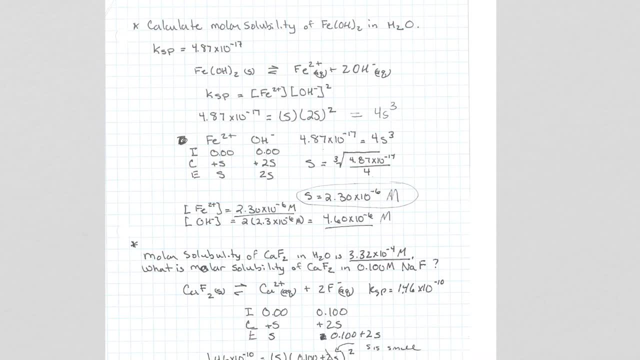 So that gives us an overview Of Solubility, equilibrium And some of the effects That we see with it Now. what I want to do now Is walk our way through A few practice problems, As we typically would do in class. 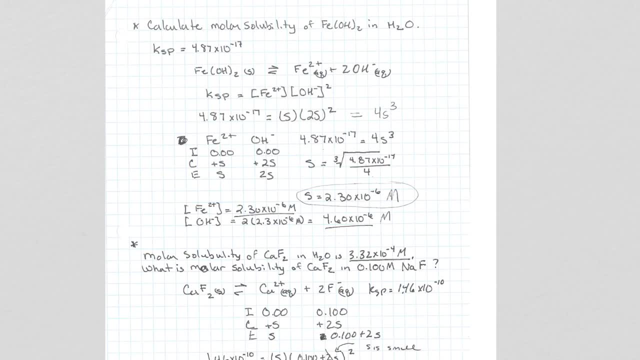 Illustrating how we can Analyze these problems Or solve these problems. So for a couple basic problems, One type of problem Will ask you To calculate The molar solubility Of some compound In water, Given it's KSP value. 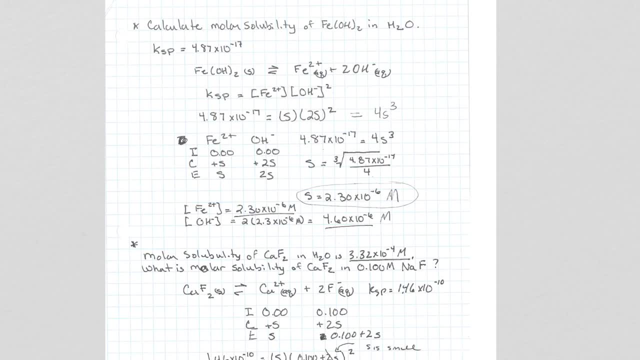 So sometimes the problems will give you the KSP, Other times, As we've seen, It won't. But you can look these up in the book. So In our example here We're looking at Calculate the molar solubility of iron hydroxide. 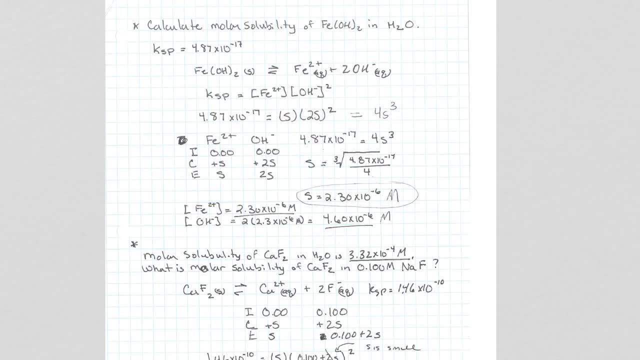 In water X 10 to the minus 17th, So a pretty low solubility. So the first thing we want to do Is we want to write out Our solubility equilibrium. So we're going to write out our reaction. 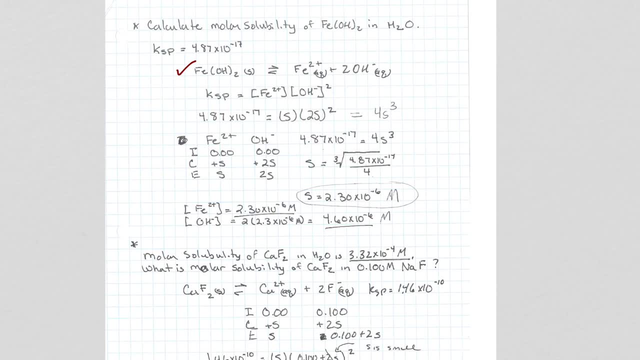 So we have our solid Always as our reactant In equilibrium With our dissolved ions Expressed at the right stoichiometry. So we're going to create 1 iron, 2 plus ion And 2 hydroxide minus 1 ions. 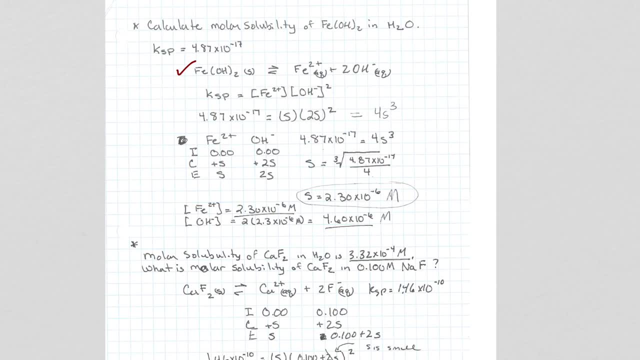 In solution We're going to write out our KSP expression. So KSP Equals concentration of iron, Times the concentration of hydroxide Squared. We plug in some numbers Now. If we looked out at our ice table here: 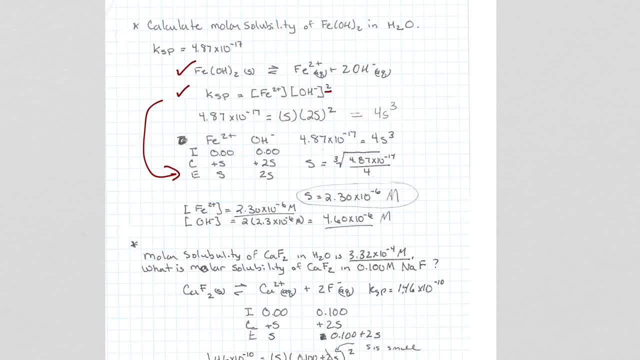 That we can set up. We have Just our products. We don't need to worry about the reactant Because it's not involved in our expression Initially, Before we add any. Our solubilities, Our concentrations, are zero. Now, instead of using X. 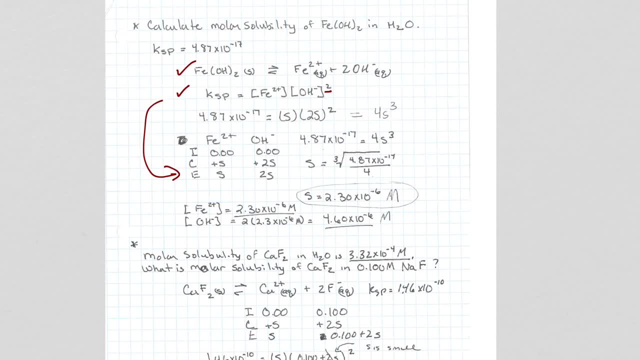 For solubility, The book will use S. It doesn't really matter, I will use S because the book does Just call it solubility Instead of using X. So When this dissolves, of course The concentration of iron is going to increase. 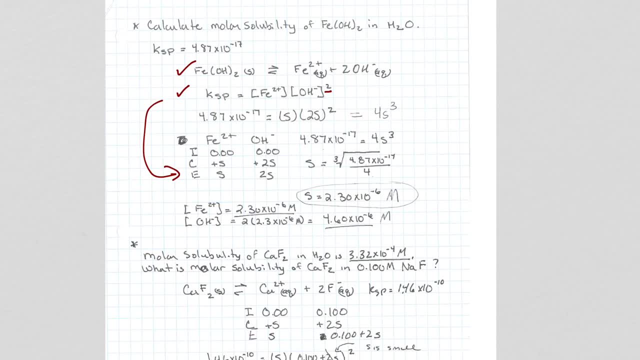 By S And Hydroxide is going to increase by 2S, So we got to make sure to keep that Stoichiometry in mind. So then, if we go back And plug these in To our expression, We have KSP. 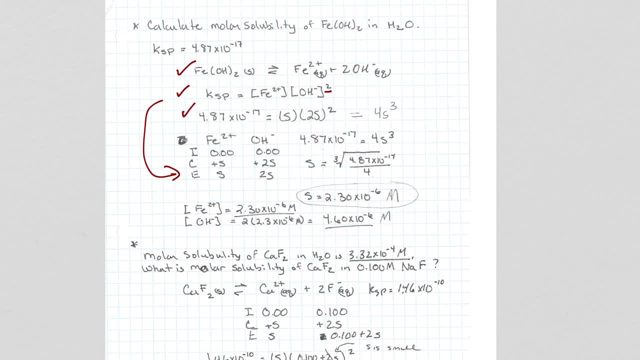 Equals S Times 2S Squared. So If we do some algebra We can reduce this Down to 4S Cubed. So 2S squared Is 4S squared Times S is 4S cubed. 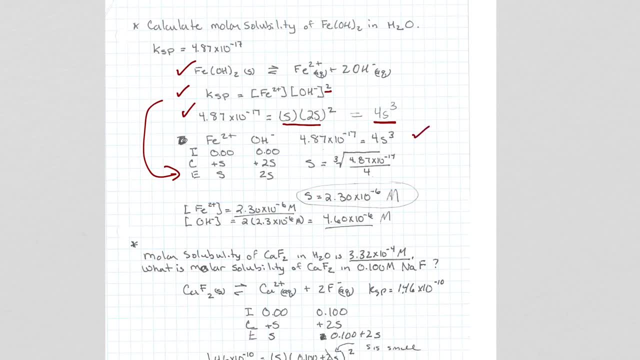 So we end up with 4.87 times 10 to the minus 17.. Equals: 4S: Cubed. We do a little rearranging. To solve for S, We would need to Take the cubed root Of KSP. 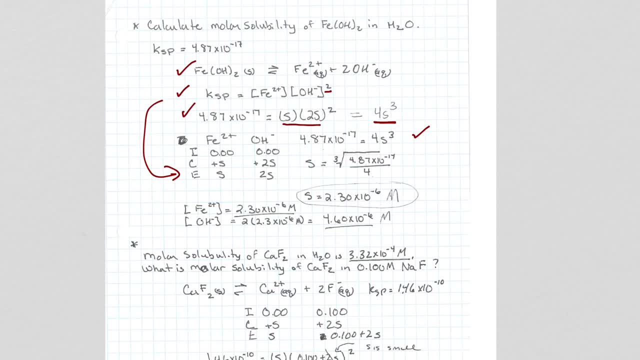 Divided by 4.. So We could do it in either order. We could first divide both sides by 4. To get a value, And then take The cubed root of that. And so We're going to take. 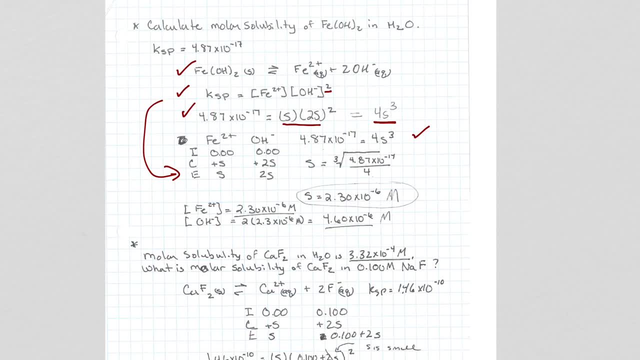 S equals the cubed root Over 4.. So We're going to solve for S And it's going to come up to be 2.3 times 10 to the minus 6. Molar Now If we then use these values. 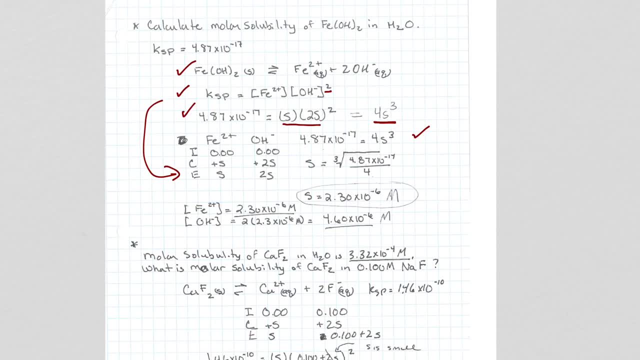 To go back and recalculate the concentrations. Well, of course iron is equal to S, So it's going to have A concentration of 2.3 times 10 to the minus 6.. And hydroxide is twice that, Or 4.6 times 10 to the minus 6.. 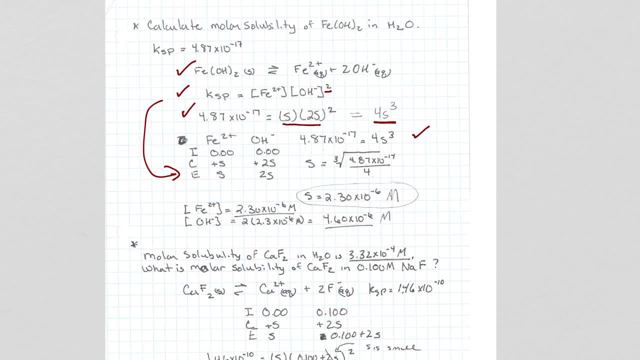 So The molar solubility, Or the solubility of these ions In solution, Is going to be 2.3 times 10 to the minus 6.. For iron, 4.6 times 10 to the minus 6.. 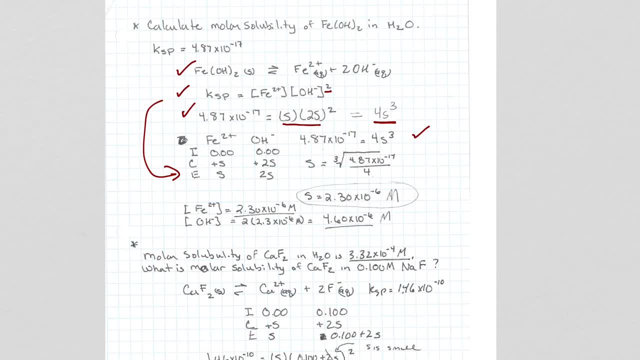 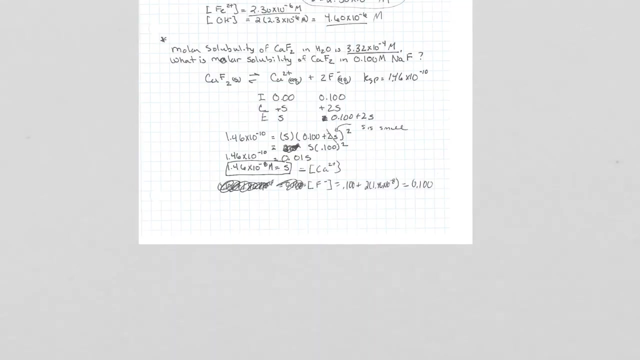 For hydroxide. Now, The overall molar solubility for the compound Itself Is 2.3. Times 10 to the minus 6.. Right, It's going to be equal To S. Okay, So that's one type of problem. 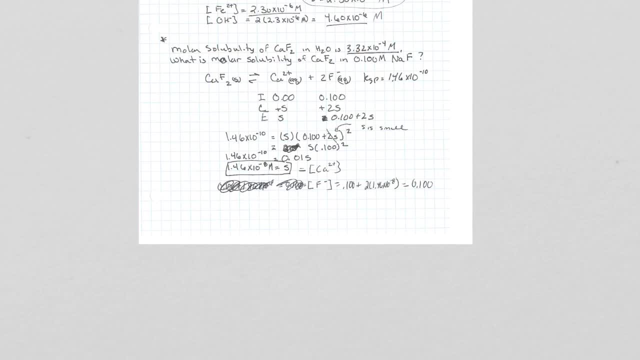 So a second type of problem Might be just the opposite: Right, Where we're given The molar solubility Of a compound And We're asked to calculate It's solubility In Common ion Right. 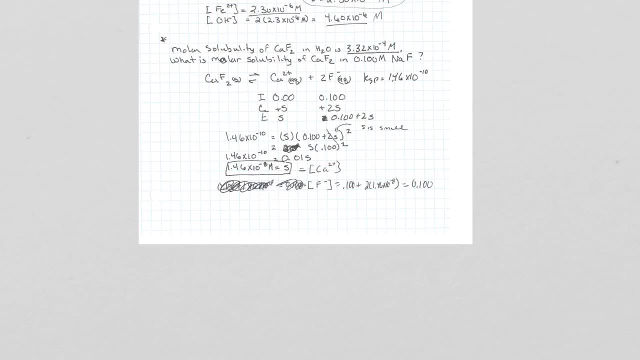 So now we're going to explore The common ion effect. So we're told that the molar solubility Of calcium fluoride In water is 3.32.. Times 10 to the minus 4.. So what is the molar solubility? 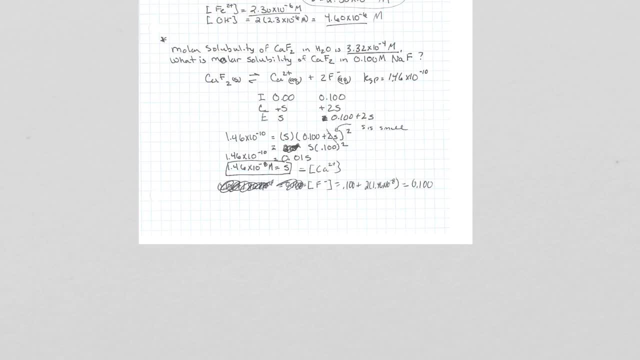 Of that same calcium fluoride. If we have A 0.1 molar, If we, instead of dissolving it in water, We dissolve it in 0.1 molar sodium fluoride Solution. So this is no different Than the problem we just solved. 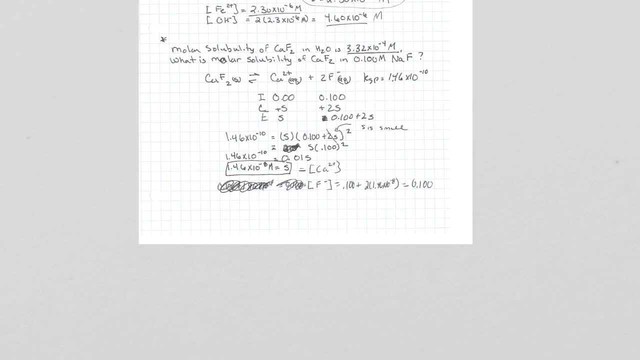 Except, Instead of having a 0. Concentration of both ions, Now We have 0. Of the calcium ion, But we already have 0.1 molar Solubility of F minus or the fluoride ions. Now the KSP here. 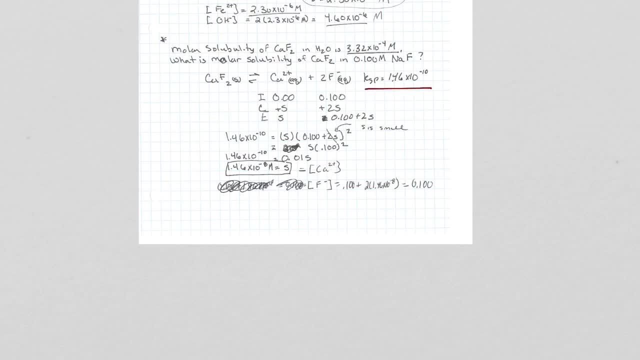 Is either given or we can look it up For this compound For 6 times 10 to the minus 10.. So we're going to Go through our ice table the same way We use our stoichiometry, And so 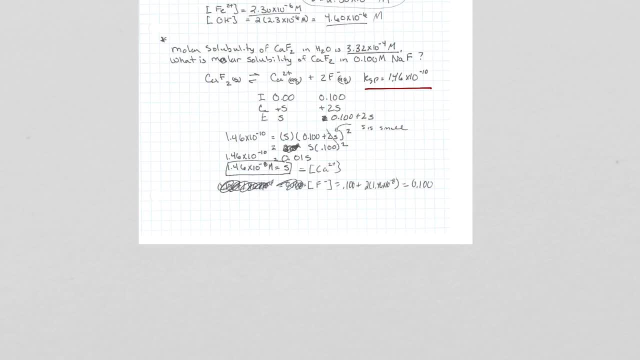 We're going to have a calcium concentration Of S and a concentration Of fluoride ions of 0.1.. Plus 2S, 2 to 1 stoichiometry. Now You'll notice the S is small Approximation here. 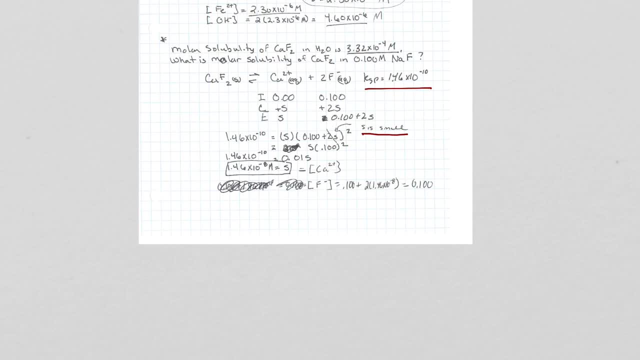 We're going to allow ourselves to make that same Approximation we have For the other equilibrium, Assuming that the change here Is not going to be significant Compared to our original concentration. So in other words, The concentration at equilibrium Is not going to change significantly. 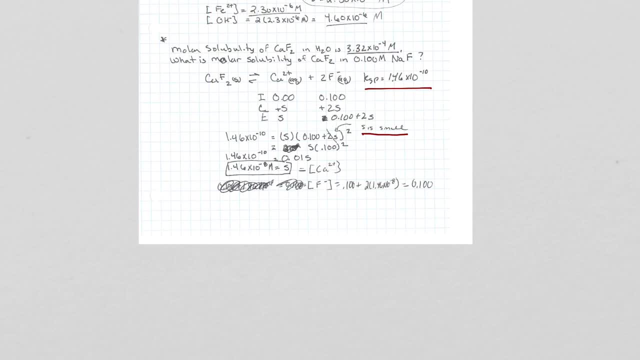 Again, that 5% threshold Is what we're going to use. So we set up our KSP. Equals S times 0.1 squared- Pretty straight forward math At this point. So S equals 0.01.. 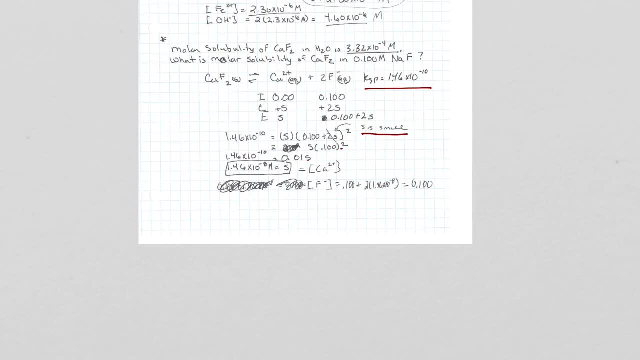 We do the square Times S, And then it's a simple division And we get: Our calcium Concentration Is equal to 1.46 times 10 to the minus 8. That's equal to S And our fluoride ion concentration. 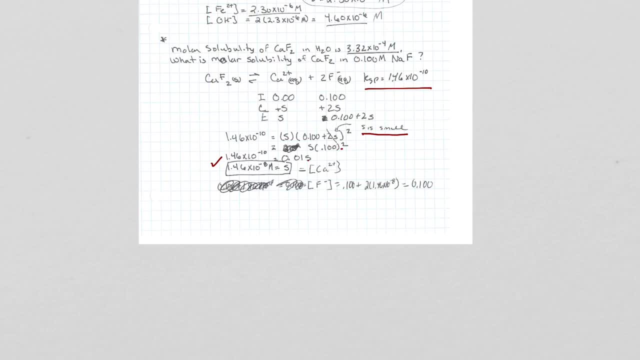 Is going to be equal to 0.1.. Plus 2 times that. If we do that, We see that To significant figures Our concentration of fluoride ion Is unchanged, So We don't really have to do the check here. 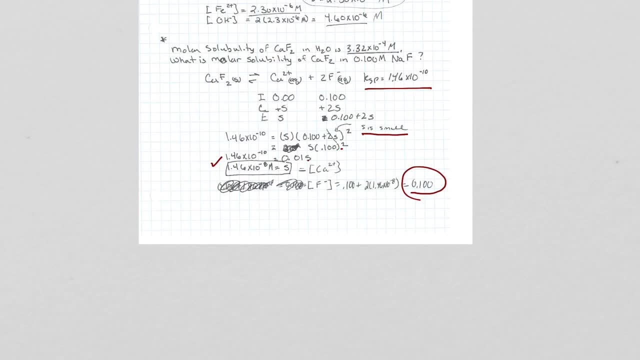 We're getting exactly the same answer And just Doing our math here, We can see that The change, The effect here Is going to be out The 0.1. In terms of The significant figures. So that's calculating. 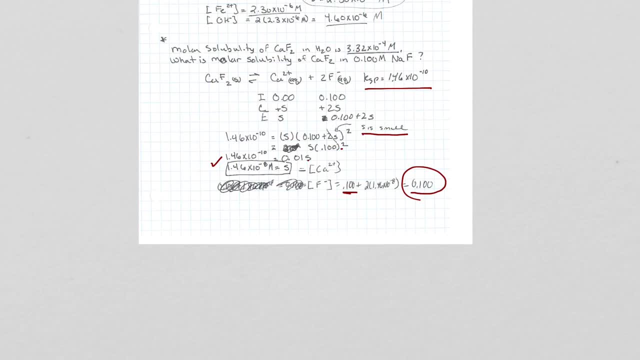 The molar solubility In a solution where We have a common ion present, And what The message here should be: that If we look at this number, The solubility of calcium Or, either words, Our molar solubility. 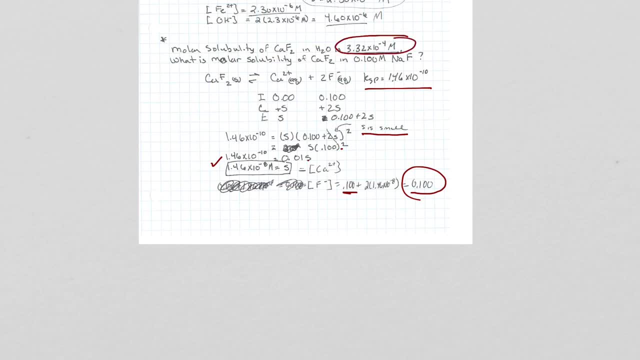 It is less than The solubility we saw in water. So in water Is 3.32 times 10 to the negative fourth molar, When we already have That common ion. As expected, We're going to push the equilibrium back to the left. 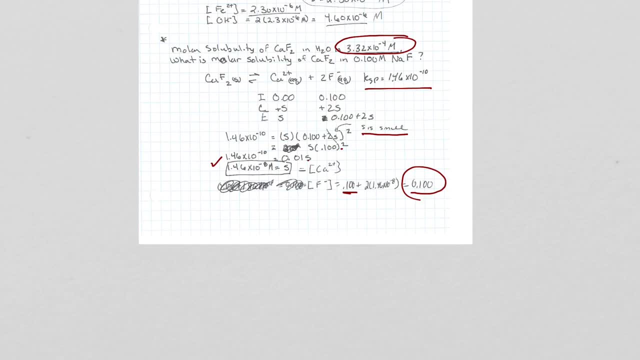 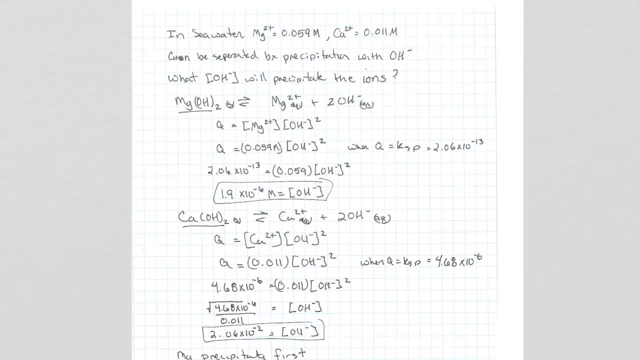 And our solubility is reduced to 1.46. Times 10 to the minus 8. So much lower solubility With that common ion present. So the last problem I want to look at here Is a problem dealing with. 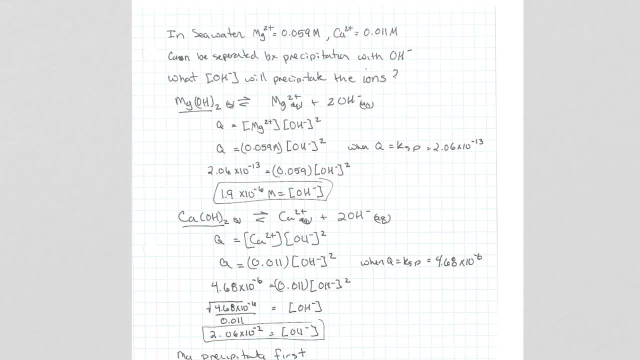 Precipitation. So our problem here is that In seawater Magnesium ions are present At 0.059 molar And calcium ions are present At 0.011 molar. These ions can be separated By precipitation. 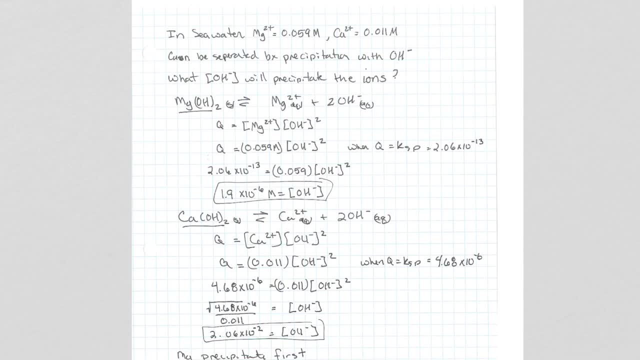 With hydroxide ion. So the question we want to look at Is what hydroxide ion is necessary To precipitate the ions. So we're first going to look at Magnesium. The concentration of hydroxide ions Would be necessary to cause the magnesium. 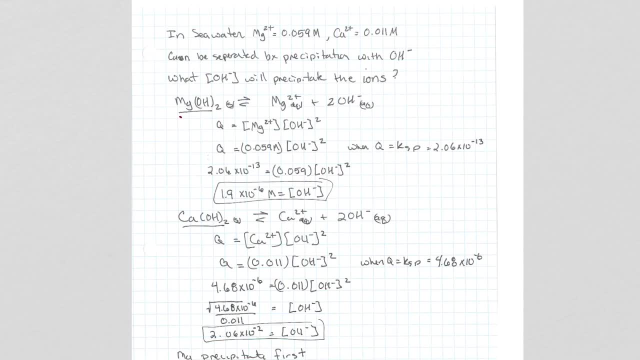 To start to precipitate out a solution As magnesium hydroxide. So the first thing is We're either given or we'll look up The Ksp For magnesium hydroxide And we see that it's equal To 2.06 times. 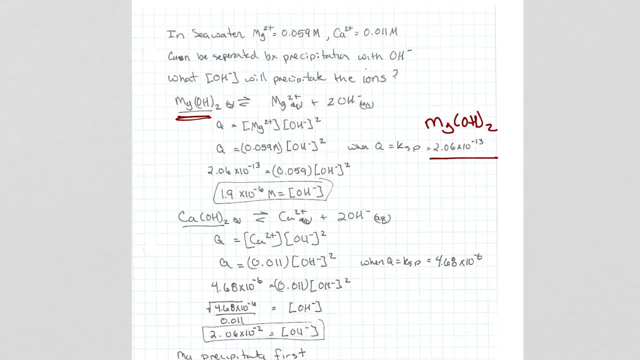 10 to the minus 13.. Now, When you're looking at the table, You might notice that That's higher or, excuse me, Lower than the Ksp For calcium Hydroxide, And what that means Is that the magnesium is going to be less soluble. 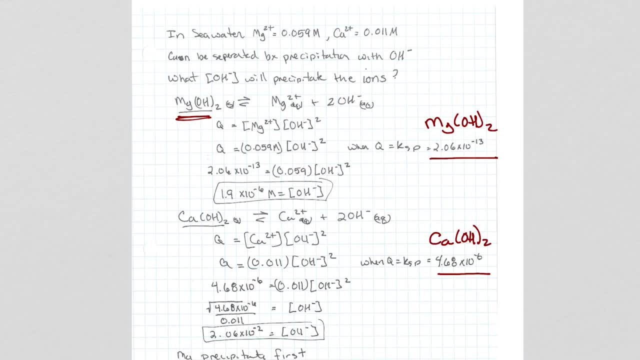 So it's going to precipitate first. So that's why we're going to look At that one first. So a reminder that That Precipitation will occur When their Q Is greater than Ksp. So what we can do 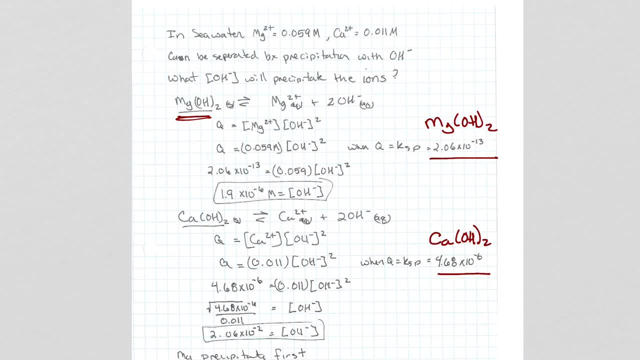 First of all Is look at When To solve for Q, At our given conditions Or at our given magnesium concentration. So in other words, We were told that magnesium Is 0.059 molar. What hydroxide ion concentration? 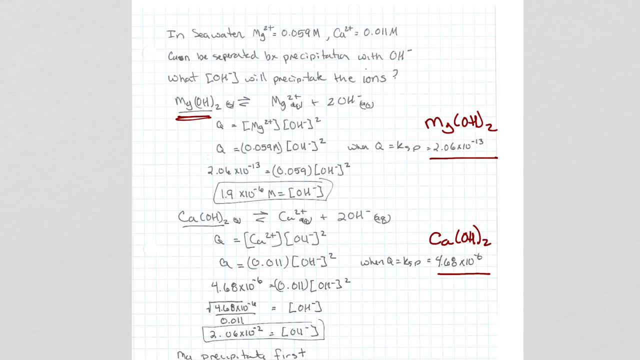 Do I need For Q To be equal to Ksp? What is my equilibrium? Concentration of hydroxide be Where we're at saturation, And so this is kind of like setting an equation Equal to 0, right? This is the point where we're going to tip. 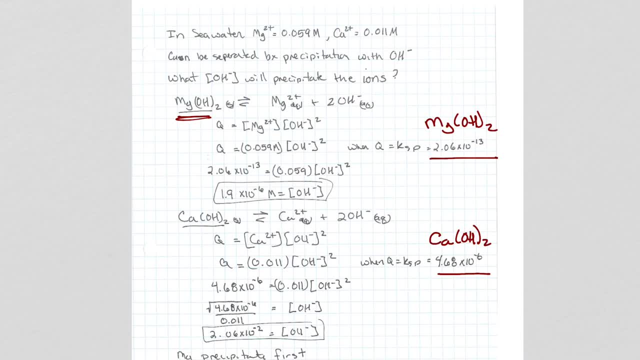 So when that hydroxide concentration gets above What we would calculate it At equilibrium Or at saturation, Then that's when the precipitation will occur. So if we solve for hydroxide ion here, Plugging in our magnesium, Plugging in our Ksp value, 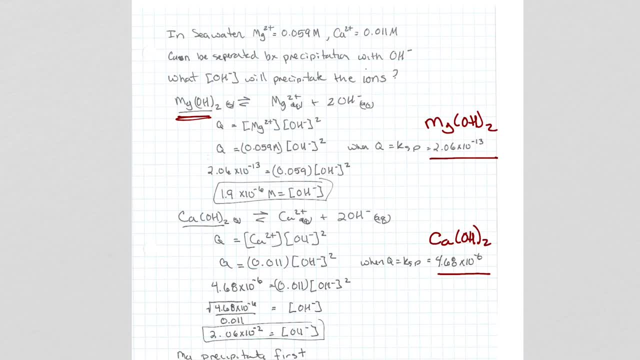 We get Ksp equals 0.059. Times hydroxide squared. We do a little algebra: Divide by, Take the square root, We get at equilibrium. Our hydroxide ion concentration Would equal 1.9. Times 10 to the minus 6.. 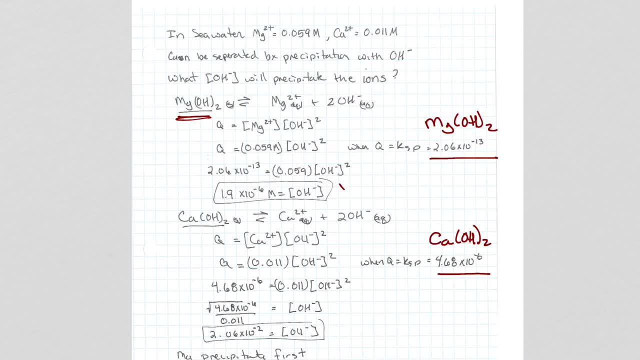 So above this. So if we're Greater than this concentration, Precipitation Will occur. So when hydroxide becomes Larger than 1.9. Times 10 to the minus 6. Then we start to get precipitation to occur. 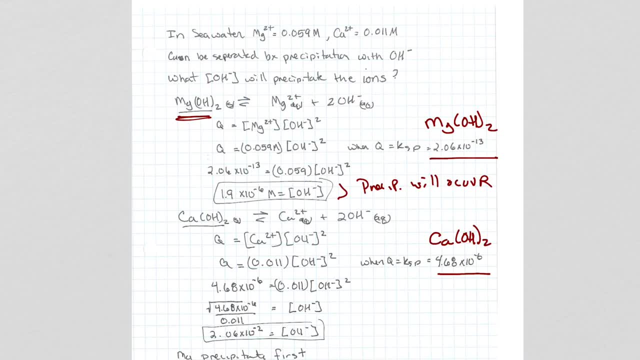 Of the magnesium hydroxide. So now, if we turn our attention To looking at the calcium hydroxide At this point, We draw out our equilibrium, Of course, And we draw out our expression Now: Our given calcium concentration. 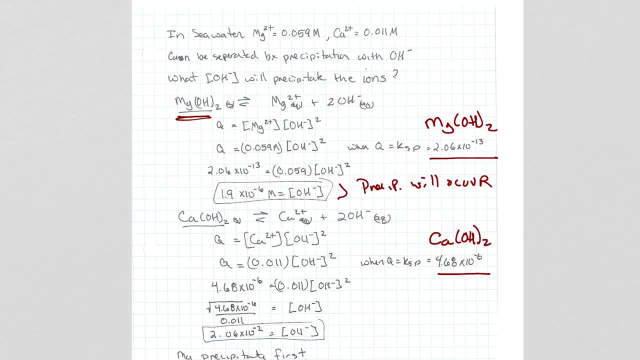 In seawater was 0.011.. And so if we take a similar approach Using the Ksp of calcium Hydroxide, We can solve for what hydroxide ion Would be present At equilibrium And therefore anything above that. 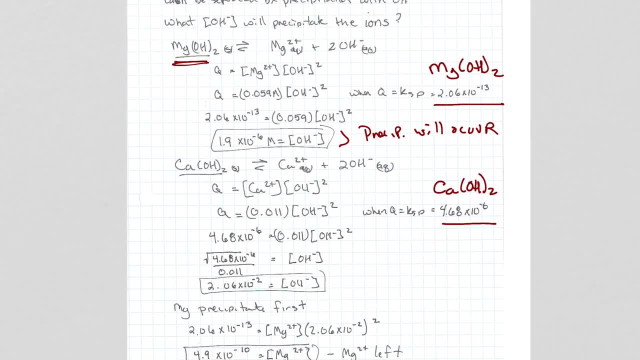 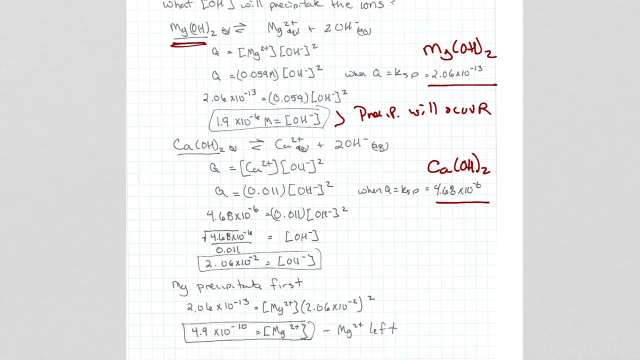 Would trigger Precipitation to occur. So if we plug it in For hydroxide ion Divided by 0.011.. Taking the square root, We get that precipitation Of calcium hydroxide Won't occur Until the hydroxide concentration. 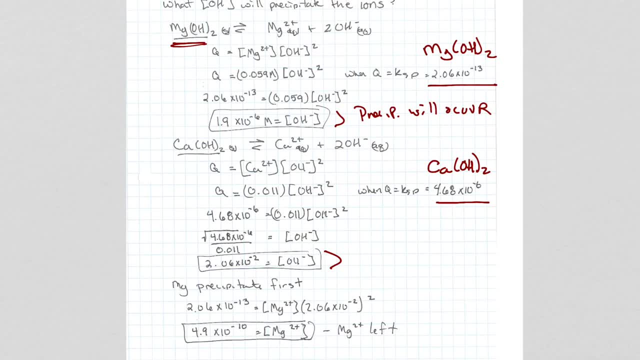 Is greater than 2.02.. Times 10 to the minus 2.. So you need a much higher concentration Of hydroxide ion To get Precipitation Of the calcium hydroxide. So what these things? What should illustrate is that 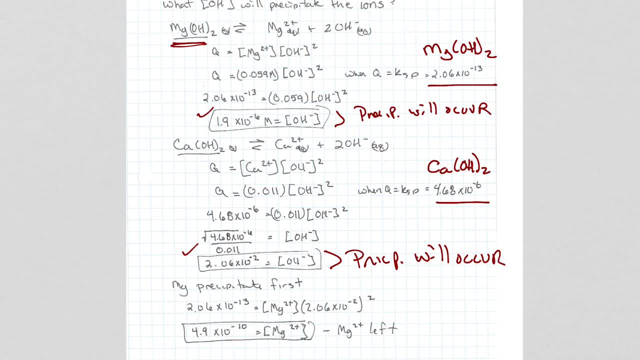 It's fairly straight forward Because there's such a big gap here, Big concentration gap, As long as we keep the hydroxide Concentration above This value And Below this value. So between these two We're going to get. 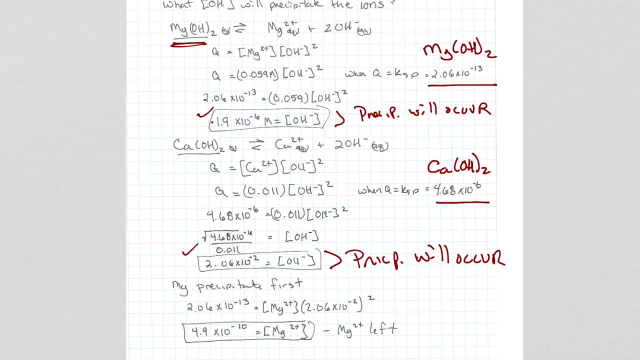 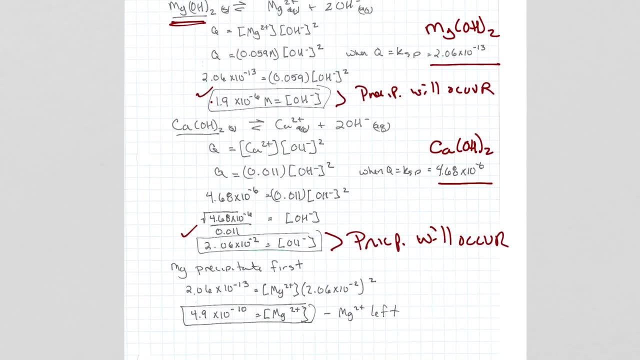 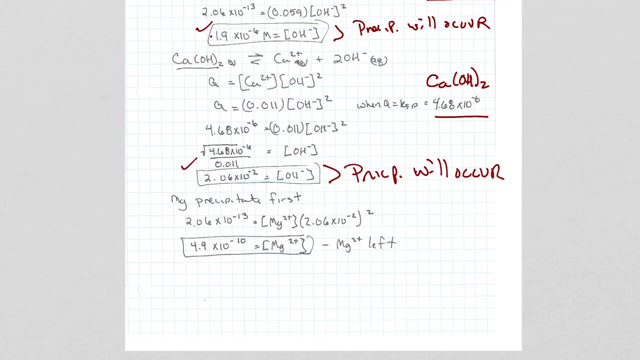 Precipitation of magnesium hydroxide. But the calcium hydroxide Is not going to precipitate, So in other words, The calcium ions Will stay in solution. So Magnesium will of course Precipitate first, And 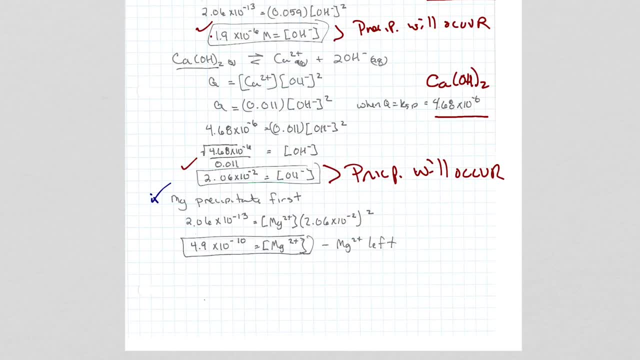 If we want to go back And see One last little thing is Okay. So we run this Here And we're going to get Precipitation of magnesium hydroxide Before The calcium starts to precipitate. So 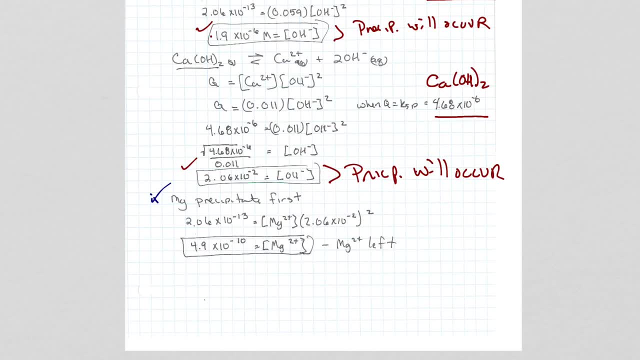 I don't want to take it beyond that If I want to keep the calcium in solution. So At this Concentration of hydroxide, How much magnesium will still be present In this equilibrium Right Now? So we plug in the Ksp value for magnesium hydroxide. 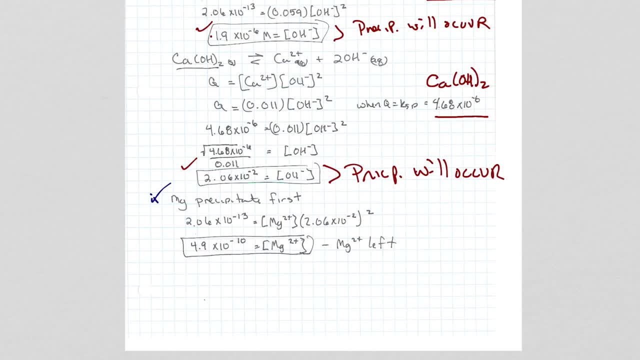 We plug in a hydroxide concentration equal to what we have before the calcium precipitates and we calculate the magnesium concentration at that point, And what that tells me is that at this point there would still be some magnesium left, at a concentration of 4.9 times 10 to the minus 10.. 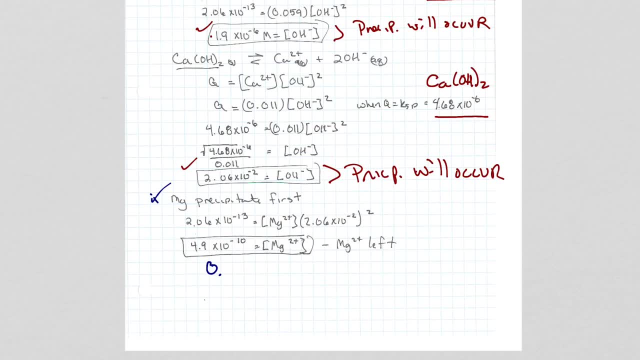 But remember our starting concentration was 0.059 molar right, or 5.9 times 10 to the minus 2, right. So we've removed almost all of the magnesium ions from solution, just leaving a very small amount in solution by adding hydroxide. 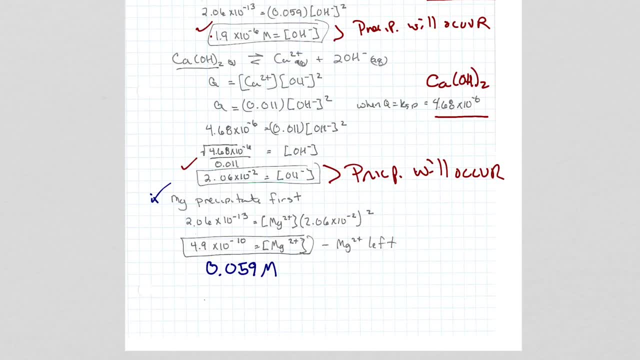 We can keep the calcium in solution, get rid of the magnesium selectively, So A use of selective precipitation. So this same type of selective precipitation that we just witnessed here in this problem is what we see with a common household problem or problem in general, especially in this. 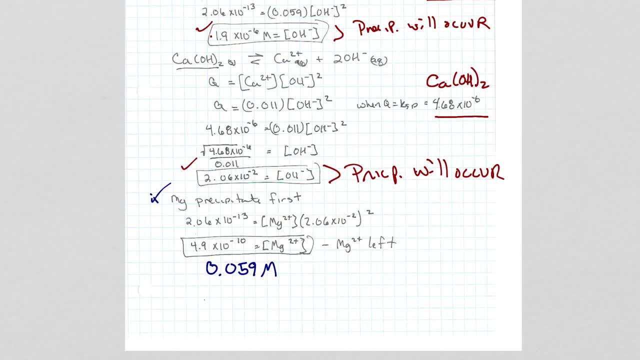 part of the country, and that is with hard water, right. So one of the things that we see is that a lot of our water has a lot of limestone in it, right, Because we have a lot of limestone in it, right. 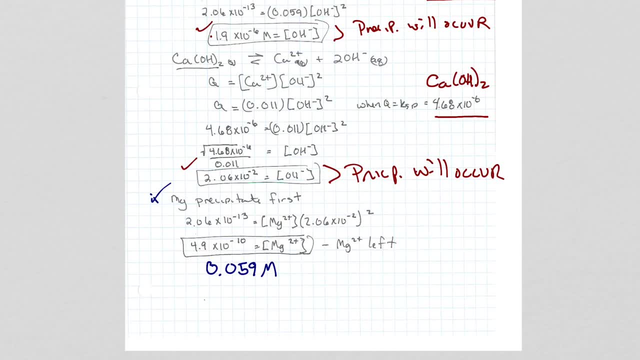 We have a lot of limestone formations and so therefore we have a lot of calcium ions. There's also going to be magnesium ions in there from various minerals, and those minerals will want to precipitate out. right That calcium carbonate and magnesium carbonate will precipitate out as the water evaporates. 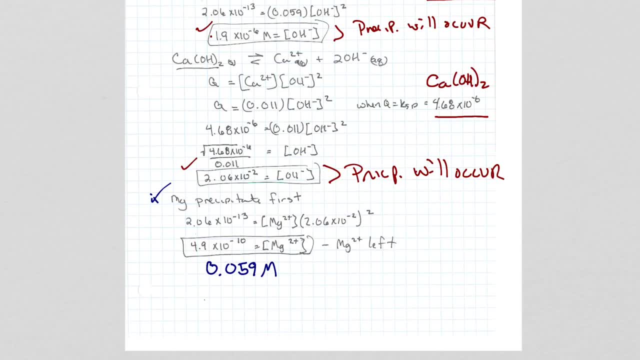 right Because they have fairly low precipitations. Now, In fact, it's exactly the opposite, in terms of order, of what we saw in the previous slide, or in the previous problem, in that, in that case, with the carbonates- that calcium carbonate- 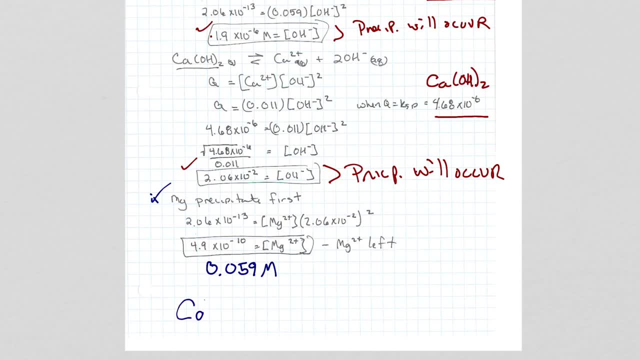 COCO3 will precipitate Right Right, Right, Right, Right, Right, Right, Yes, Yes, Yes. And also an folks' Cin defense: Kalau horses over right, I want to всп caste that was. 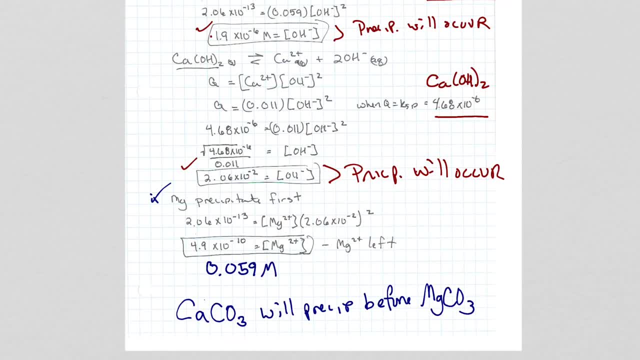 So what is COCO3?? COCO3 is an toxin that's in small particles and the part of it is called the limestone right And it's somehow well marked, or marked, And also, as time goes on, punch into more. in smaller particles, the larger molecules. 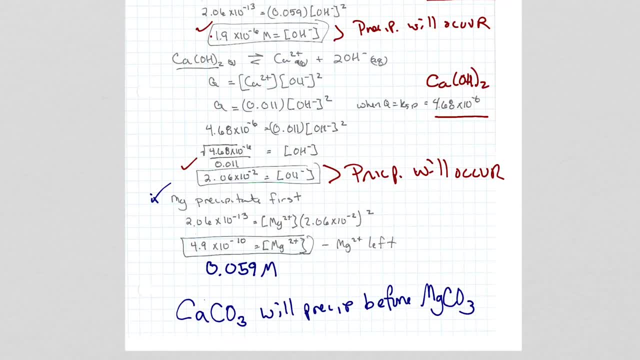 mix together that roleTS bios이� histoire갈 を 물GrM. So you get these on, you get. you get water spots. or you get water drops left on showers, on drains, on in tubs, right. The water evaporates. If it contains these compounds, well, then they will tend to precipitate out and not stay dissolved and leave spots behind. 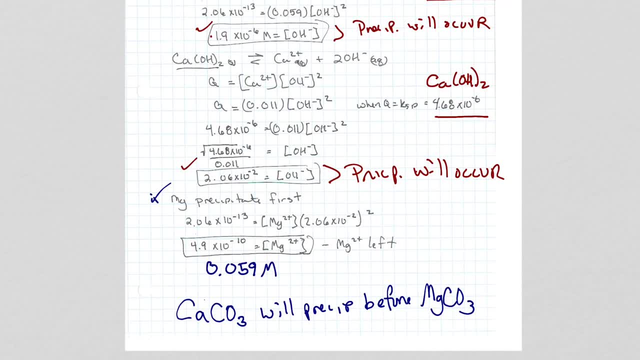 Right, Well, we call hard water spots or hard water deposits, And of course, these can build up over time in pipes and on different faucets and so forth, And we see these hard water buildups Now. this also links back to something we saw earlier. 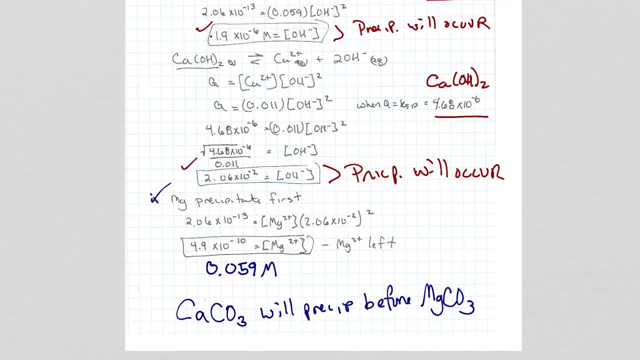 And that is why do we have all of this calcium carbonate in solution. Well, if we think back to our earlier discussion on pH solubility, or pH effect on solubility, we saw that under acidic conditions, that materials, that these compounds, become more soluble. 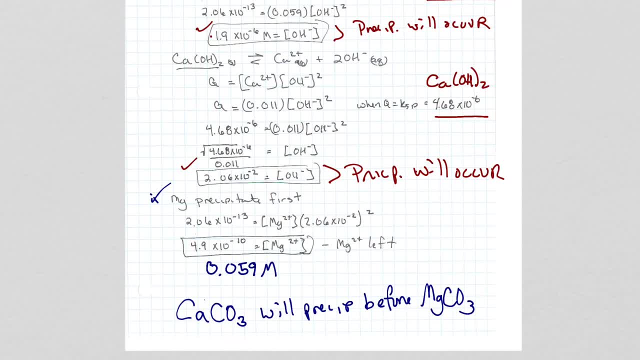 So if we have limestone and we have rain, right, rain, as we remember, tends to be acidic And so a lot of times water, natural water, is soluble. But if the limestone is slightly acidic, just because of rainwater being acidic, it will tend to dissolve or the limestone will tend to become dissolved in this. 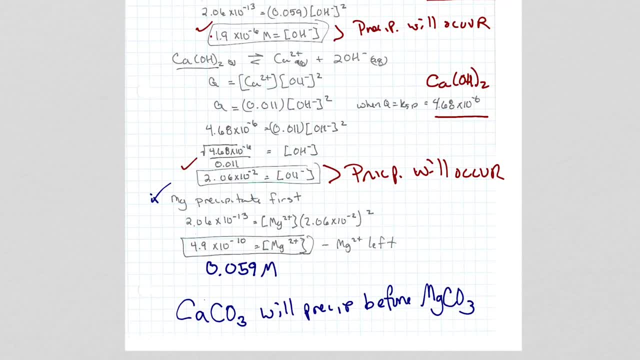 And this will lead to high concentrations of carbonate and calcium ions in solution. This also leads to some interesting natural rock formations, of course, because, as this saturated Materials are said to, water that's saturated with calcium carbonate starts to drip or starts to form right we get the formation of stalactites and stalagmites in caves.